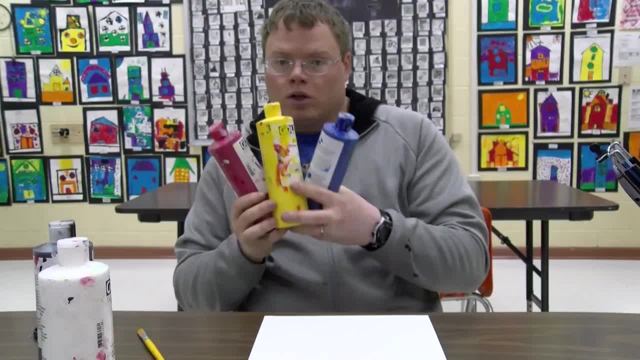 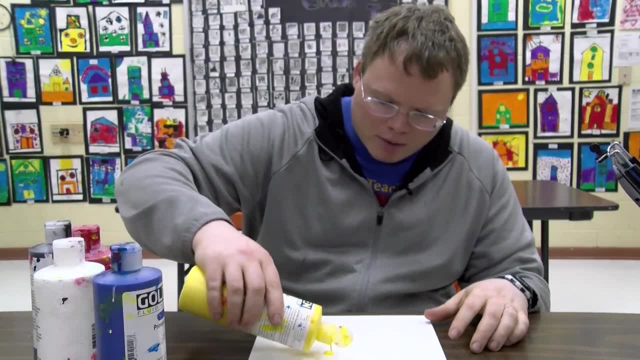 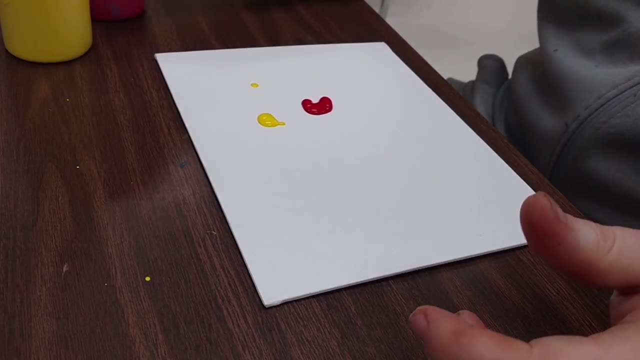 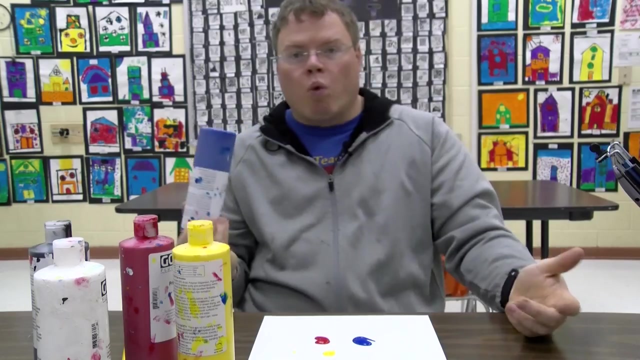 The first important thing to learn about color is the primary colors, which are different when you're talking about pigment than they are when you're talking about light. The primary colors are yellow, red and blue. Why are they called the primary colors? 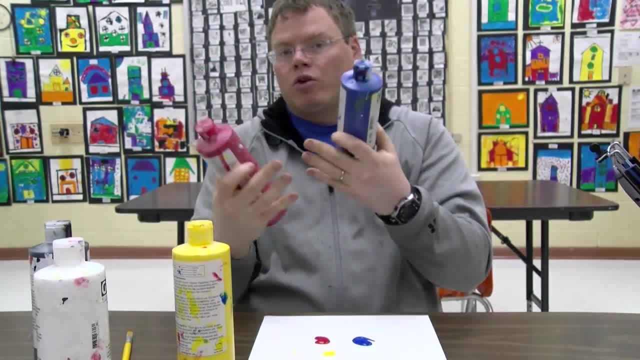 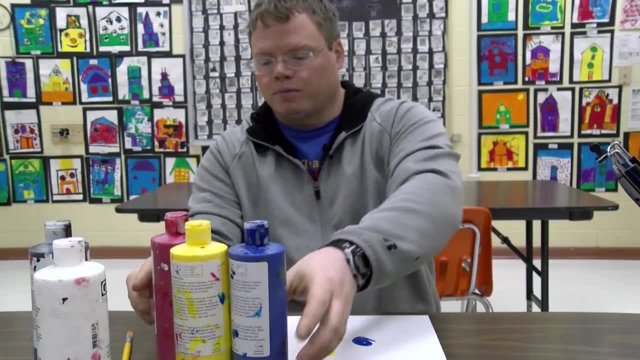 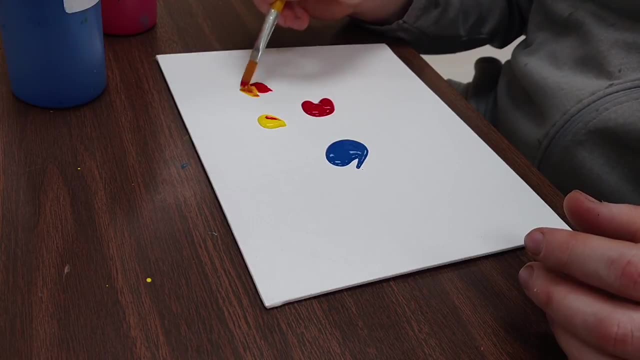 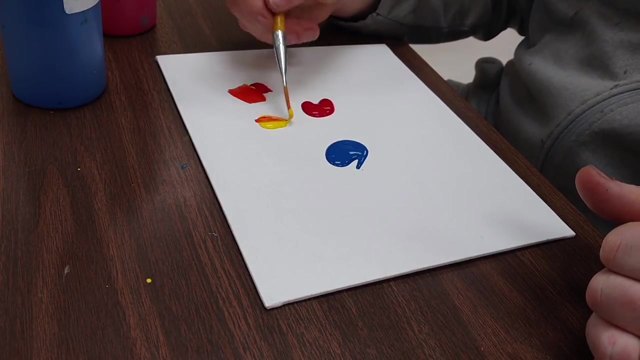 Because any two of these colors can be mixed together to create a color. You can create a secondary color, but you cannot mix other colors together to make the primary colors. For example, red and yellow mix together to make orange. The more yellow you mix, the brighter the orange will get. 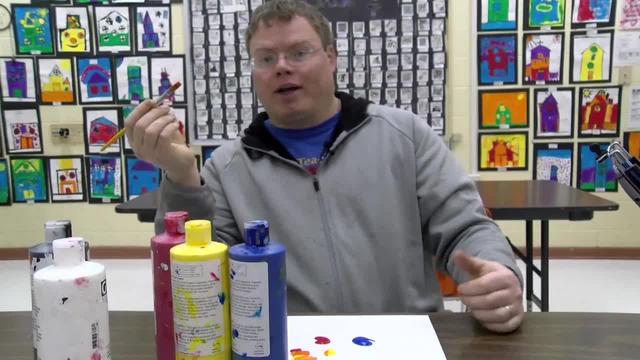 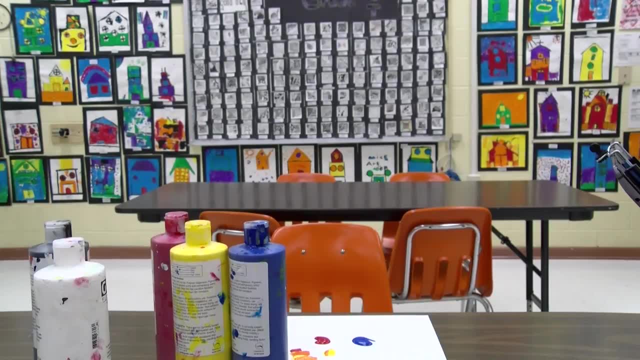 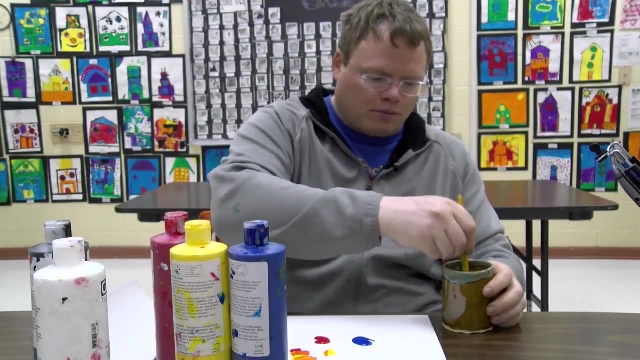 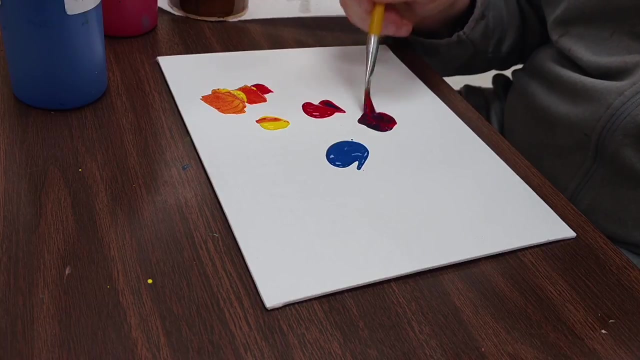 I totally forgot to get a cup of water. I've got to go rinse my brush. Okay, now I'm actually ready to get started And I just spilled some water on myself. Oh well, I can also mix blue and red to make a purple. 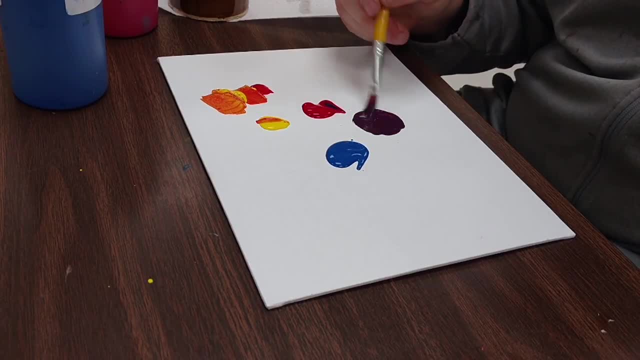 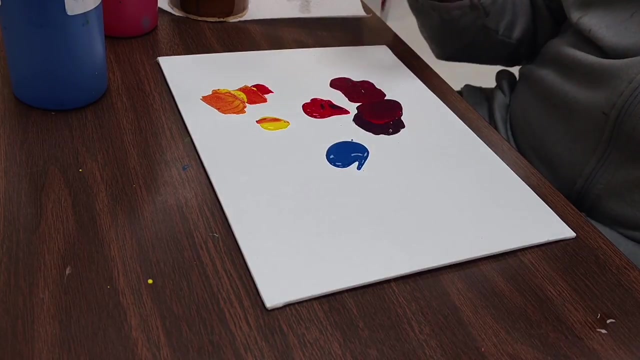 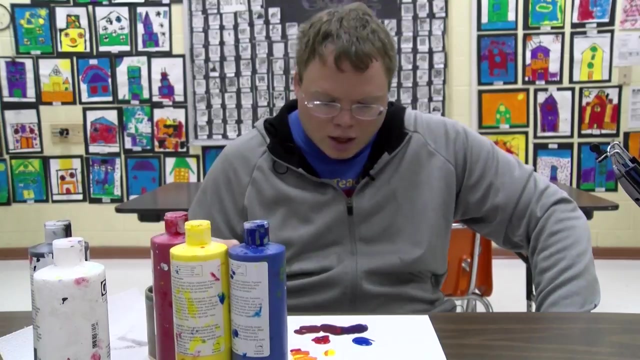 The more red I mix, the warmer that purple becomes. The more blue I mix, the darker the violet will become, And mixing more blue makes it a deeper, darker, bluer violet Again. rinsing my brush And finally I can mix blue and yellow together. 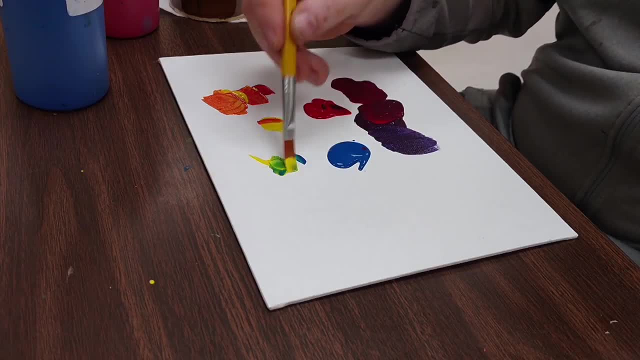 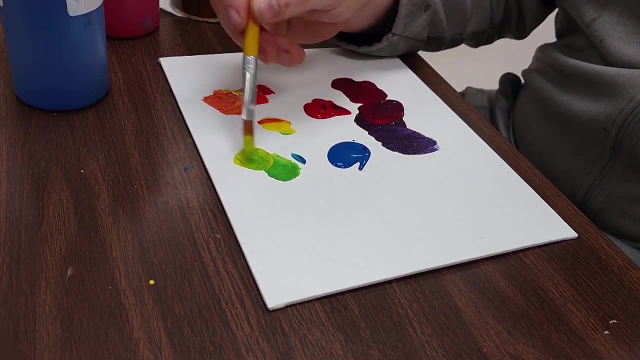 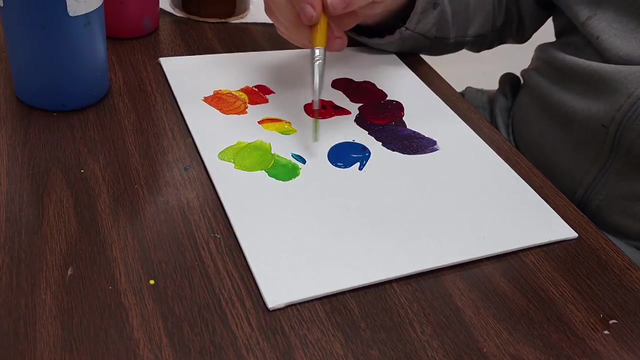 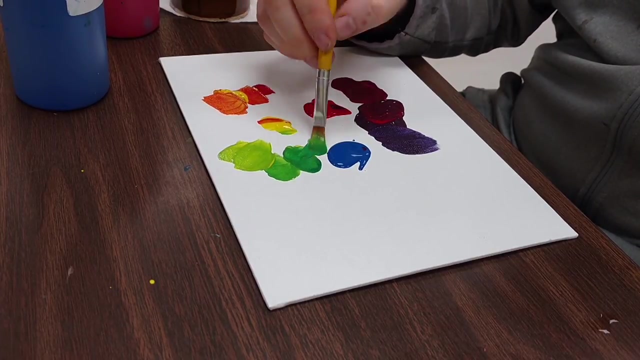 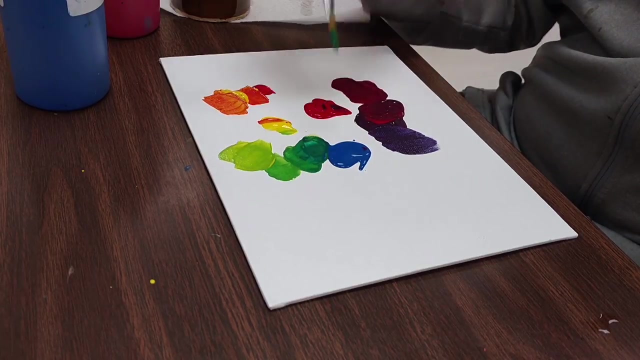 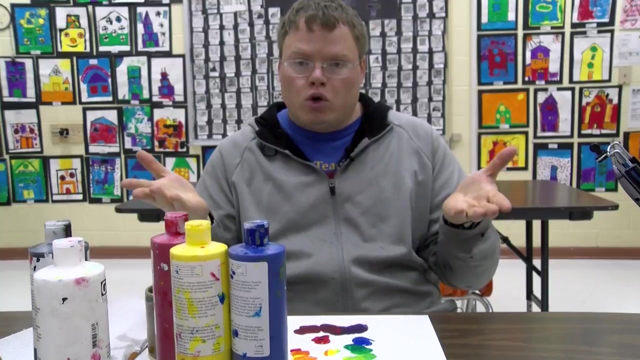 to make green. The more yellow I mix with that green, the paler, limer green I get, and the more blue I mix with that green, the more of an aqua, turquoise, teal green I get. So what we've just discovered is a word called hue, The hue of a color. 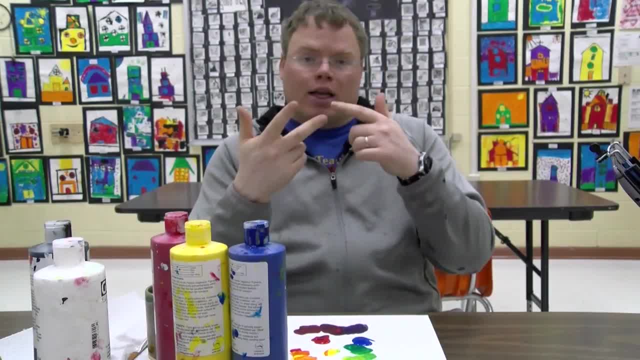 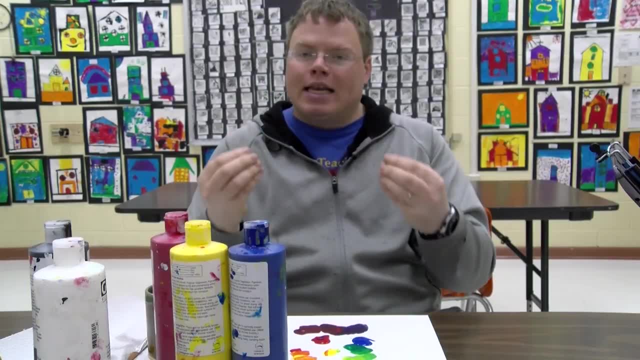 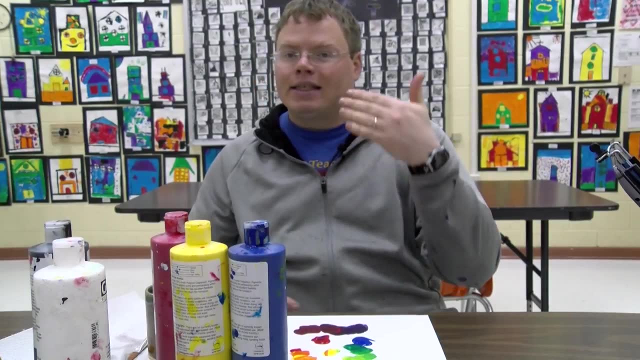 tells us what the name of the color is. Is it red, yellow, blue, magenta, turquoise, fuchsia, lime, green? It's the name of the color. It tells us where on the color wheel it is. The second thing we need to learn about color is its. 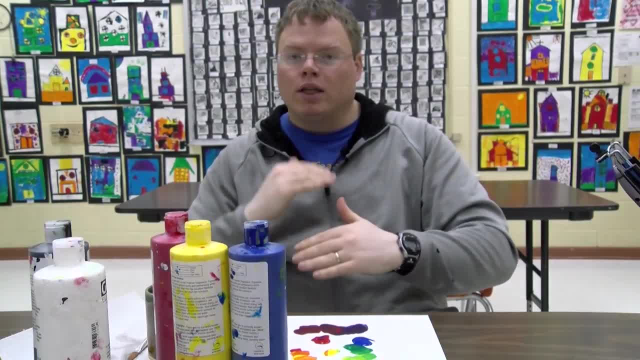 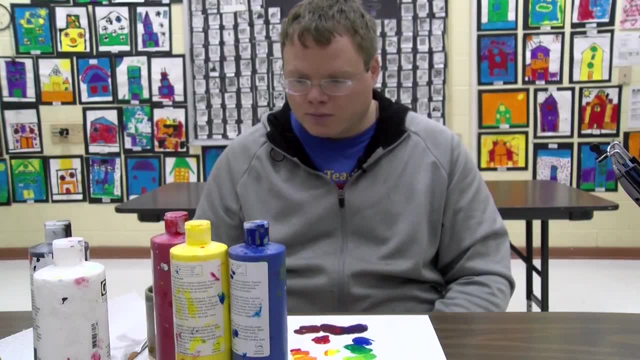 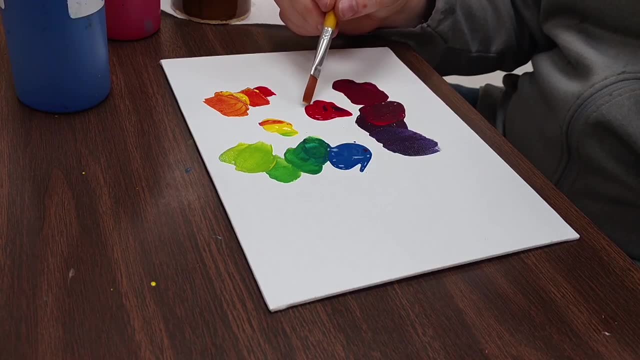 saturation, which is how much color or how little color is in our color. So what I can do to desaturate a color is mix the opposite on the color wheel. Here I have some greens If I mix a touch of red, just a tiny touch. 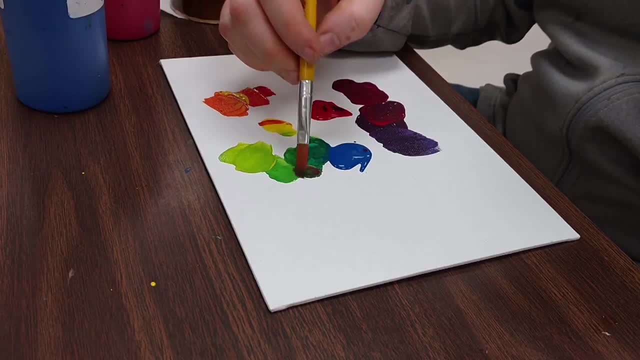 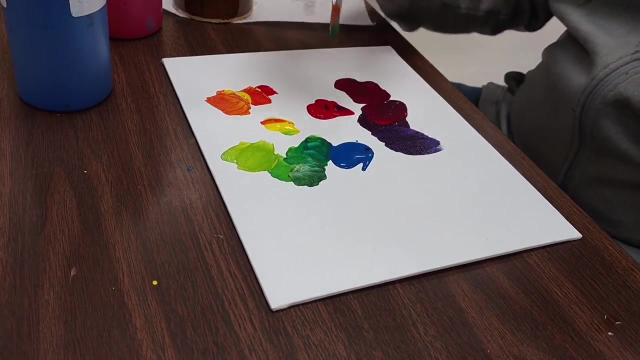 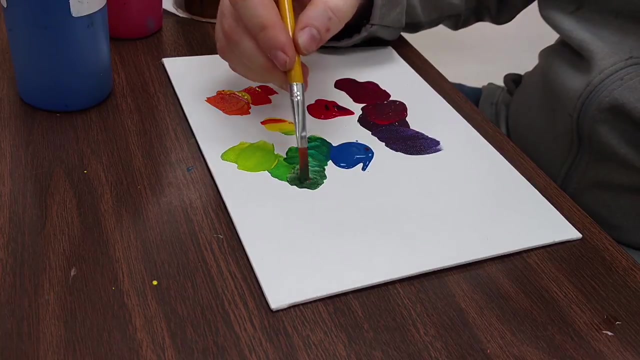 of red into that green. it will turn it into a more brownish color. It desaturates the green. It takes some of the green out of the green. By using opposites on the color wheel, we get a browner version of the color. But what if I want a grayer? 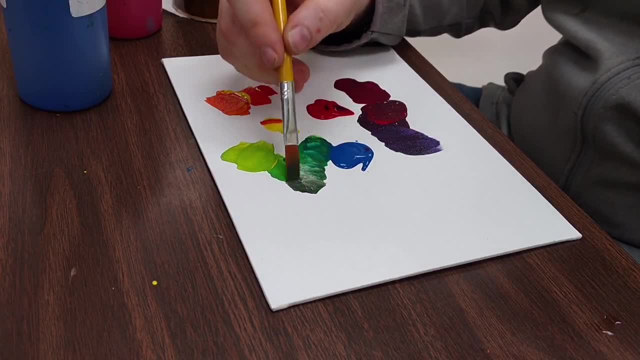 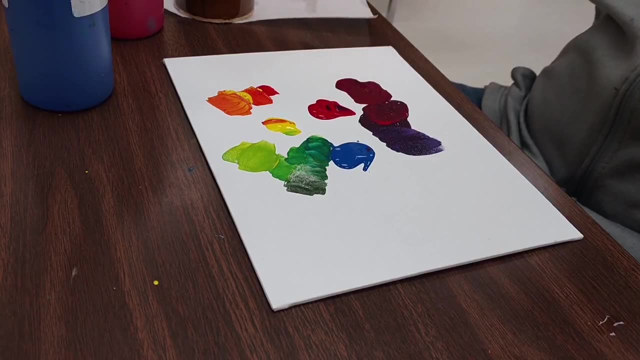 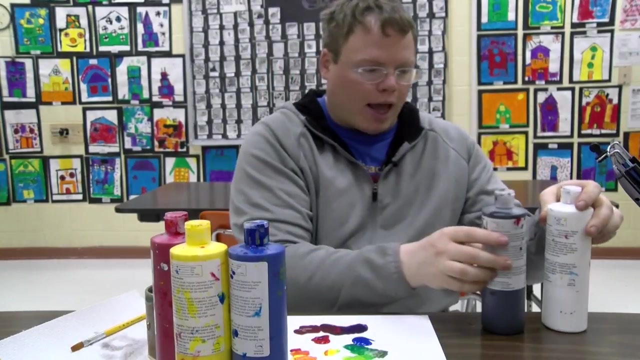 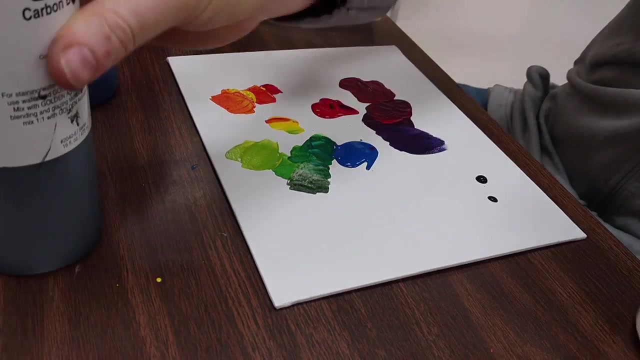 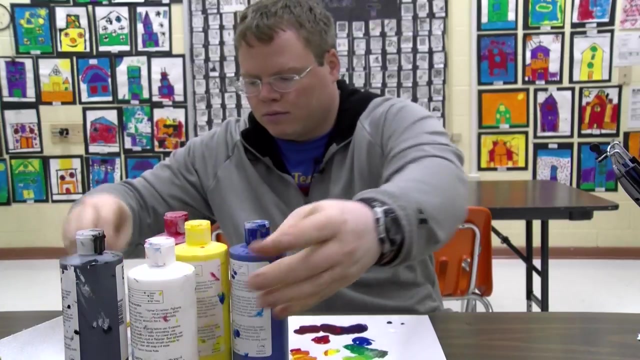 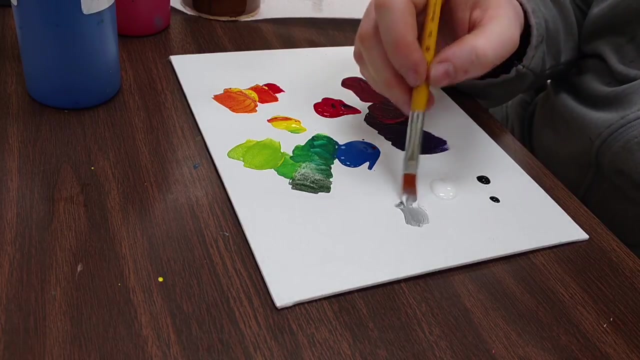 version of the color Gray and brown are both considered neutral. So there, I've created a brownish green by mixing red with it. To create a grayish green, I need some gray. I'll mix black and white. So I'll start by figuring out what value of gray I want, how light or dark I want that gray to be. 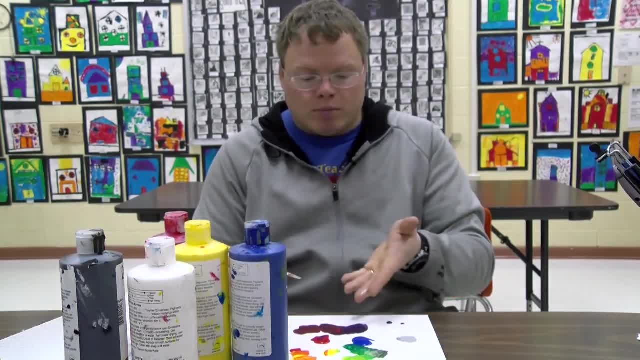 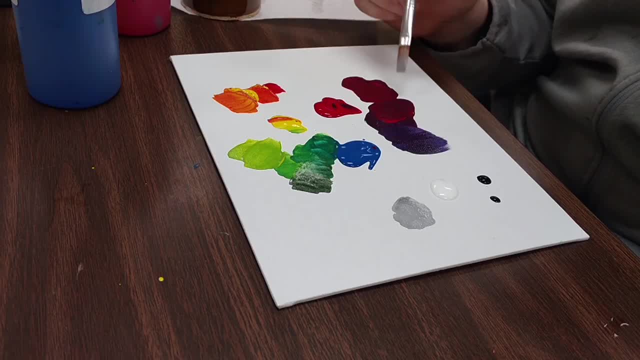 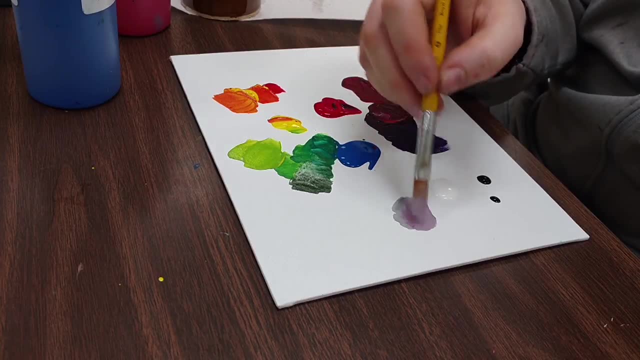 And then I can mix any one of my colors with that gray To make a grayish neutral tone of that hue. So let's say I want to take this red violet color from here and make it into a grayish red violet. I can mix it with that gray. 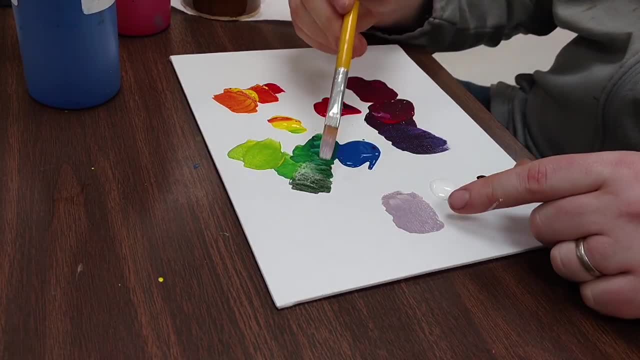 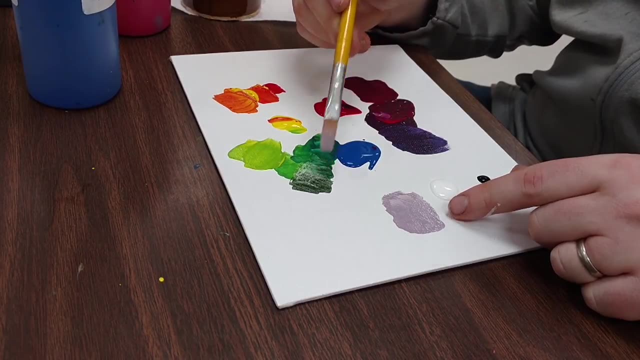 That's another way to desaturate the color. So there I've got two different desaturated colors- One I've made it more gray and one I've made it more brown- And the last thing I want to do is talk about value. 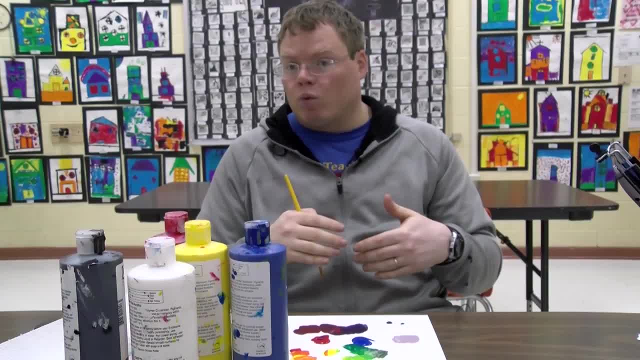 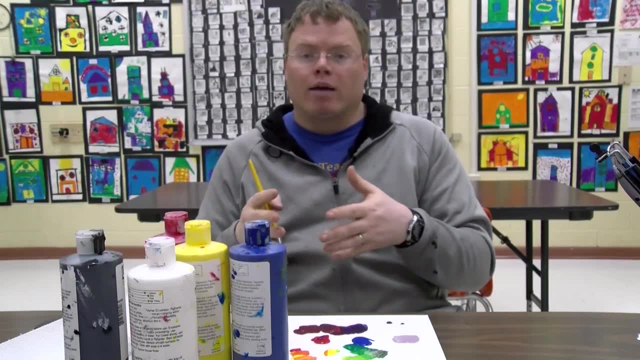 Which I kind of hinted at just before there when I was talking about the black and white making a gray. But I can change the value of a color as well. instead of just making a gray value, I can make a lighter or darker version of a color. 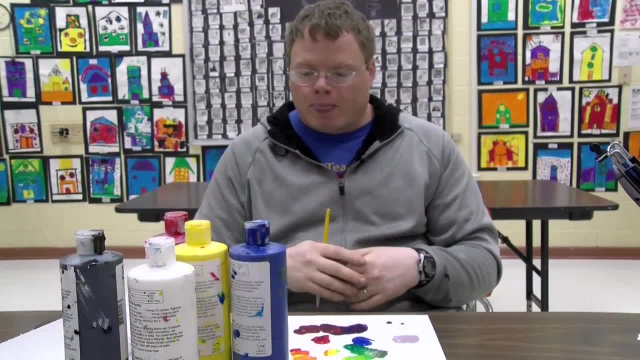 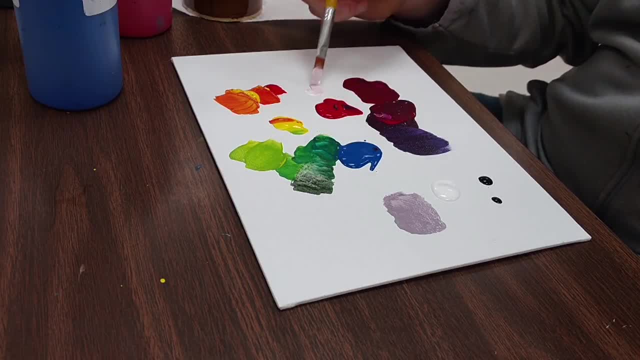 Those are called tints and shades. A tint is when I mix white with a color such as red to make a lighter version of that color. So here I've made a pink By mixing white and red, One of the things that bugs me a lot of times in my classroom. 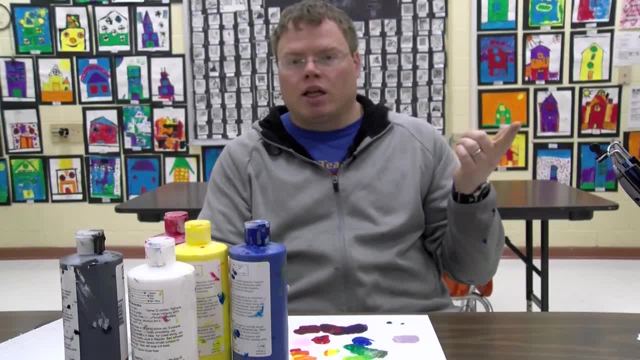 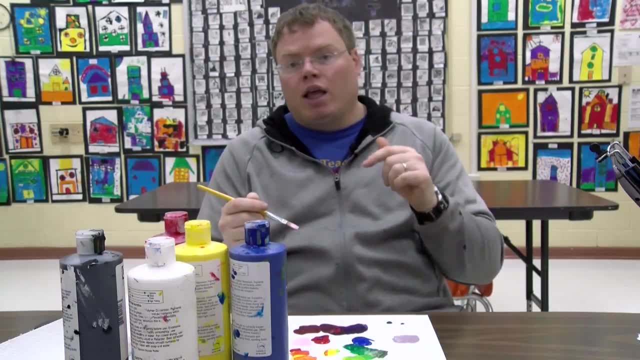 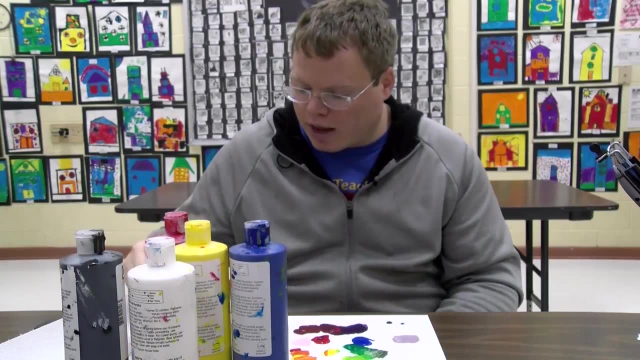 Students will say pink is a shade of red. No, it's not. Pink is not a shade of anything, It's a tint of red. Pink is red plus white. A shade is a color plus black. So let's see what that would look like. 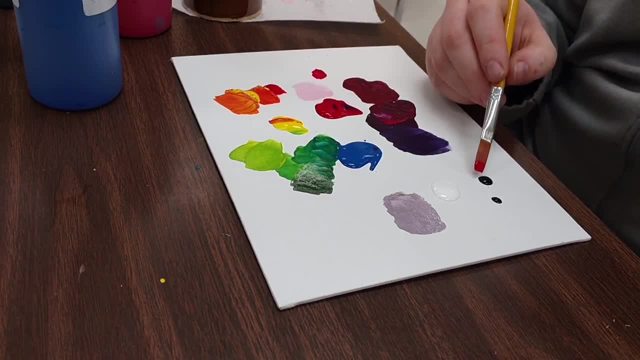 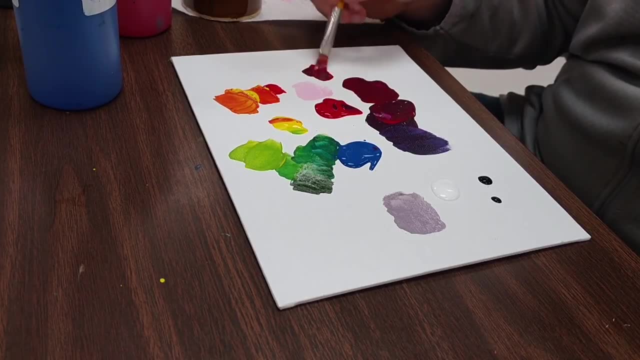 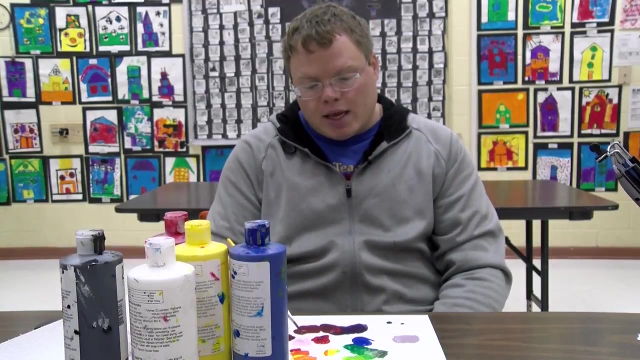 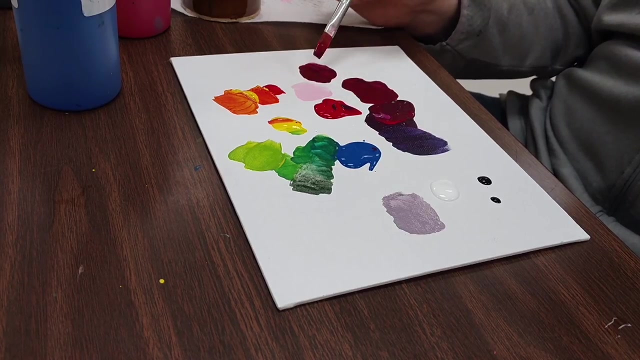 If I want to make a shade of red, I would mix a tiny touch of black with it to make it really dark, A dark maroonish kind of red. Now you notice that making a tint or a shade also changes the saturation. My pink and my maroon are both less saturated than my vibrant red there. 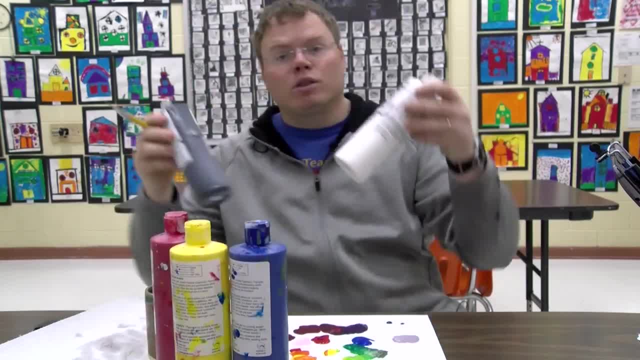 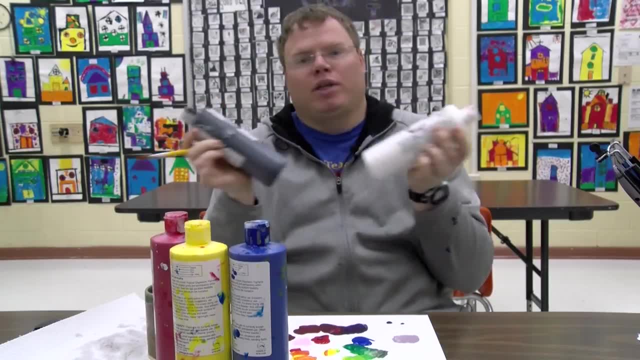 But they are also a different value. Now it's important to also understand black and white as colors themselves, Because you know there's a big debate. A lot of people will say black and white are not colors And a lot of people say, yeah, it's, black and white are colors. 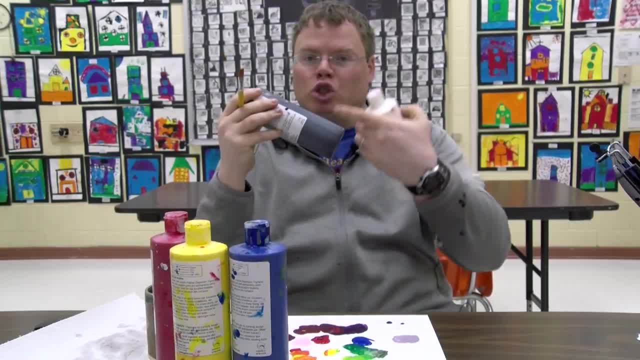 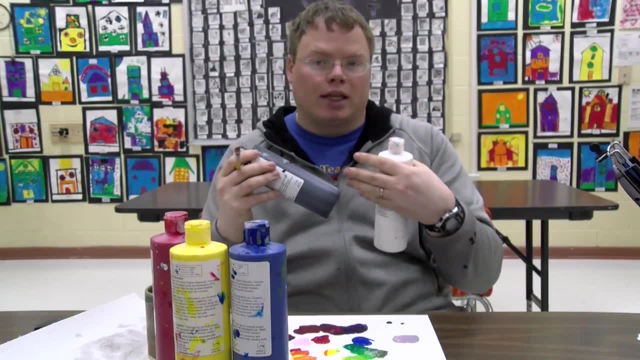 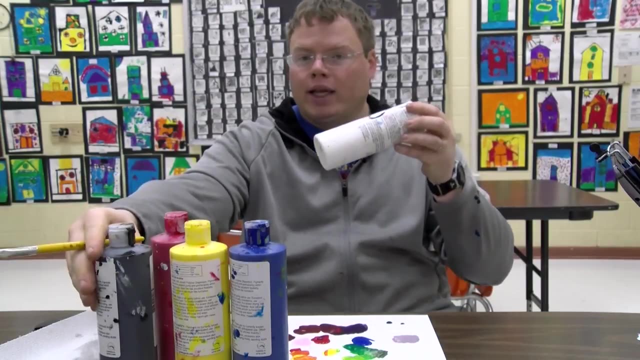 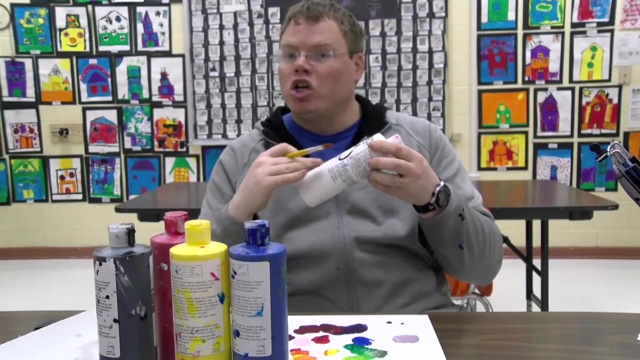 In pigment. black absorbs all the different wavelengths of light And reflects very, very little light, So you could say that it is acting like all of the pigment, And white does the opposite. It reflects all the different colors of light And so it acts like none of the pigments. 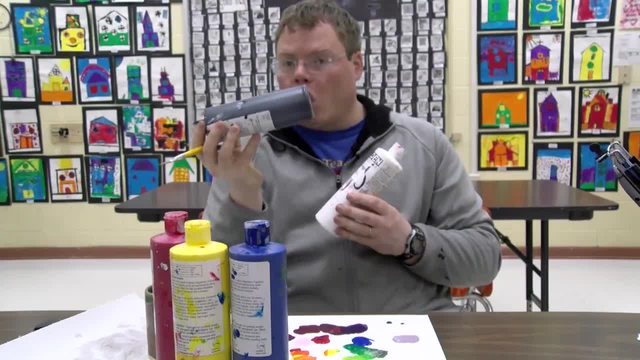 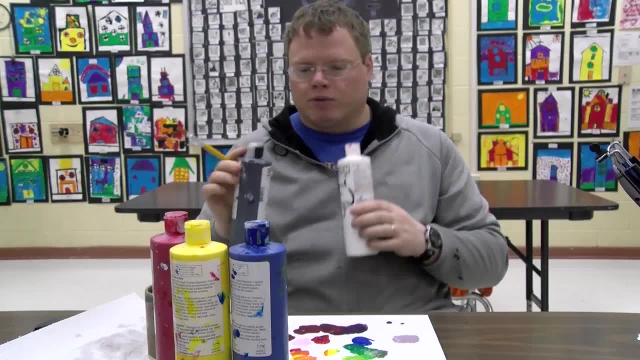 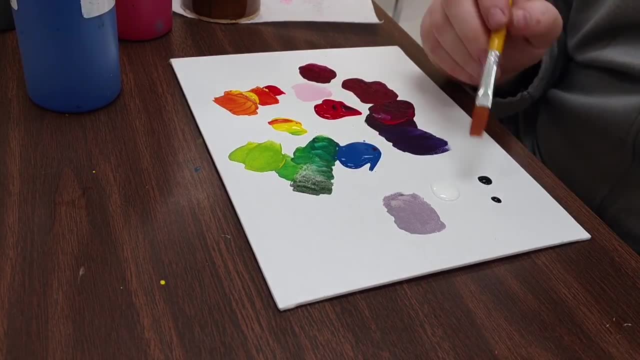 So you could say black is all the colors and white is none of the colors. The opposite would be true if we were talking about light, But that's a whole different story Here on my canvas here I have some white and some black, And let's think about those as 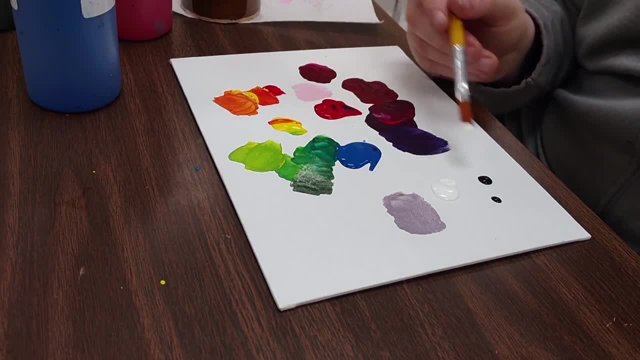 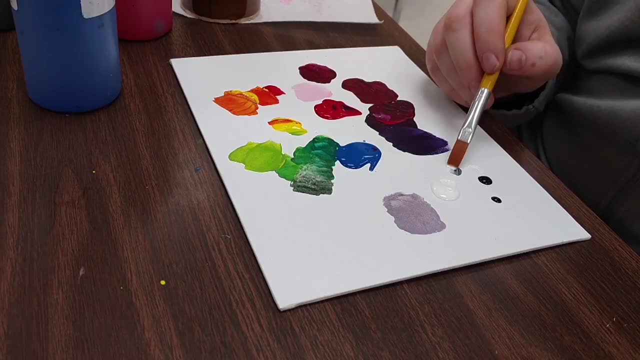 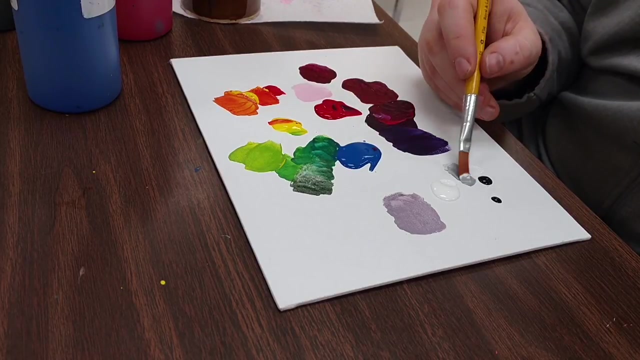 Colors themselves, Because the way that they interact with each other- Black next to white- Is super high contrast And also the way that they mix together Can affect each other and all the colors around them. So if I mix up a gray like this, 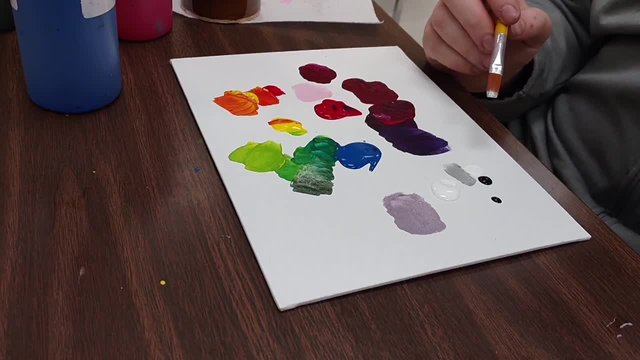 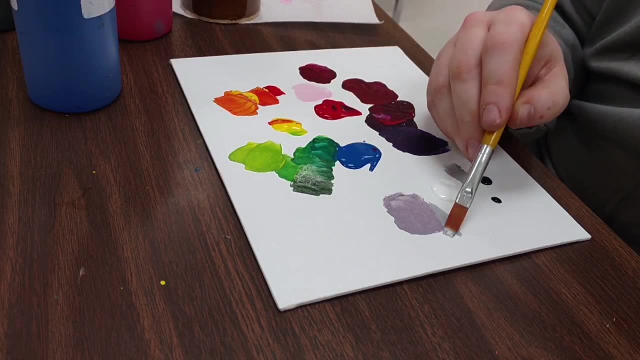 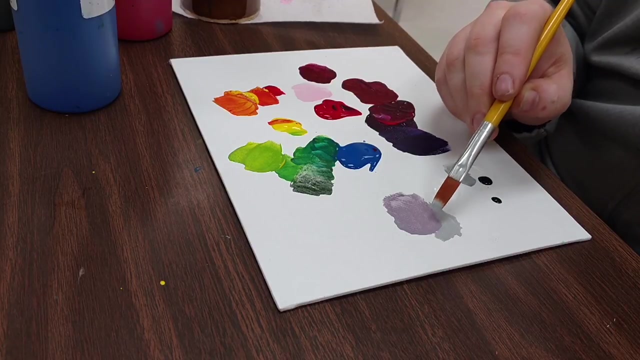 That is a completely neutral value. There's no color in it, No other pigment in it, And if I put that next to one of my desaturated colors, It makes that desaturated violet color Look more saturated than it was by itself. 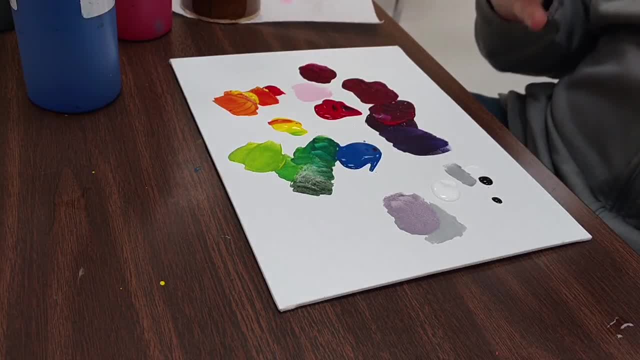 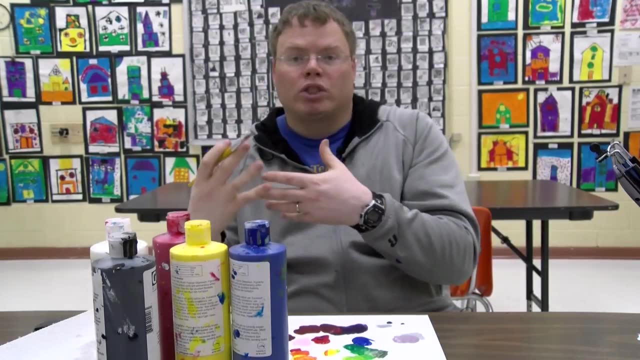 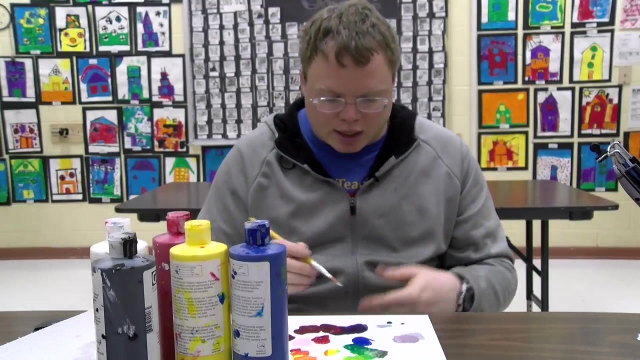 So the way that colors interact with each other Is: if you have a neutral color Next to a more saturated color, Then it will make the more saturated color look Even more saturated. So what does that mean? Let me take this gray again. 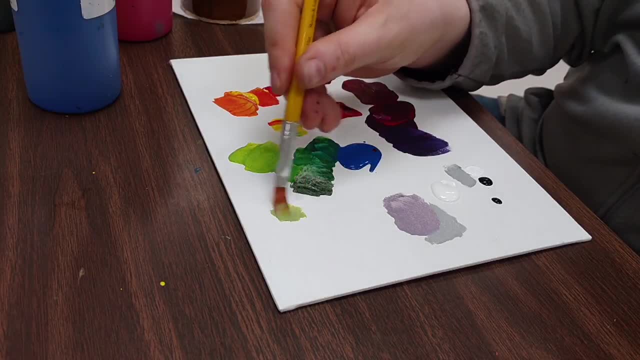 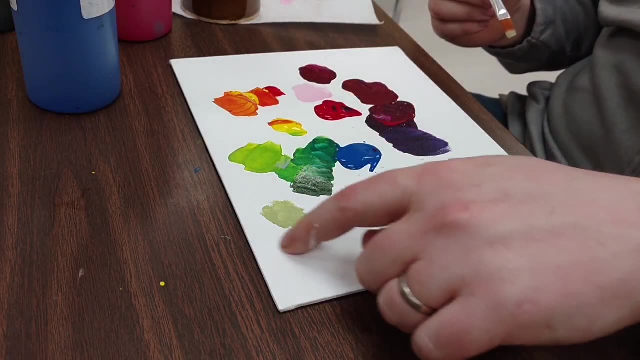 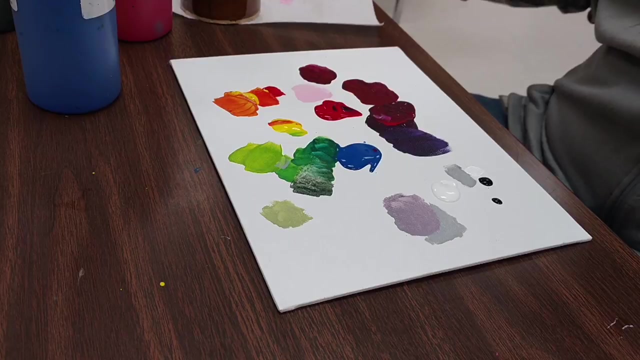 Mix it with. I don't know, Maybe some of the green Maybe make a desaturated green here. That desaturated green When it's surrounded by white, Which is a neutral color. Or if it was surrounded by gray, Let me get a gray. 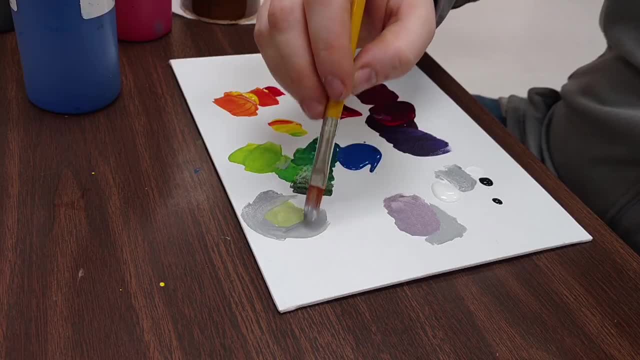 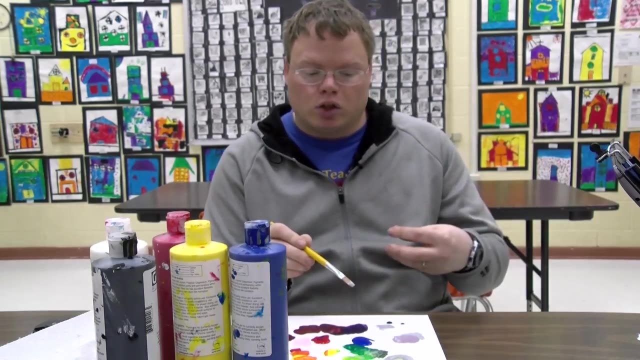 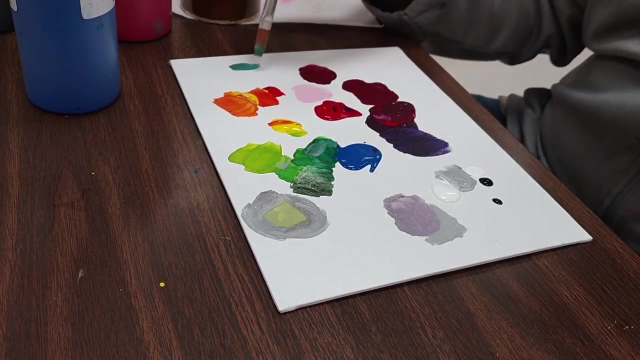 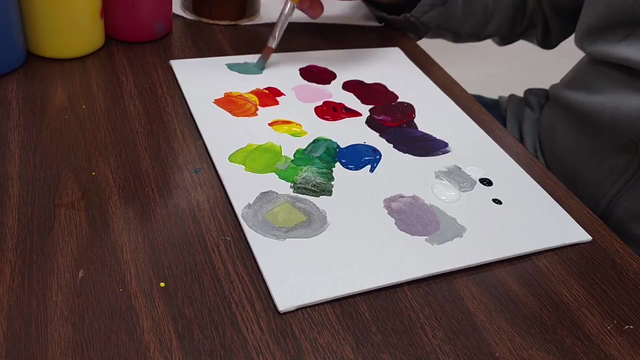 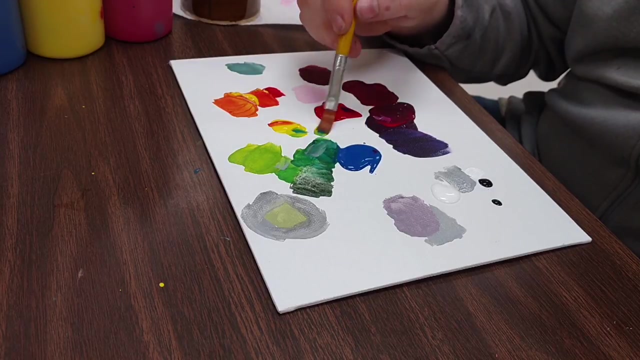 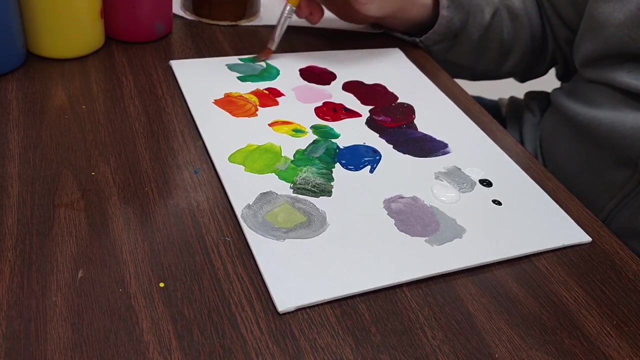 Because it's surrounded by a neutral color, It looks quite a lot more green than it actually is. But if I take a desaturated blue green here And I surround it with a very saturated green, A very saturated color, Like Like a very saturated blue green. 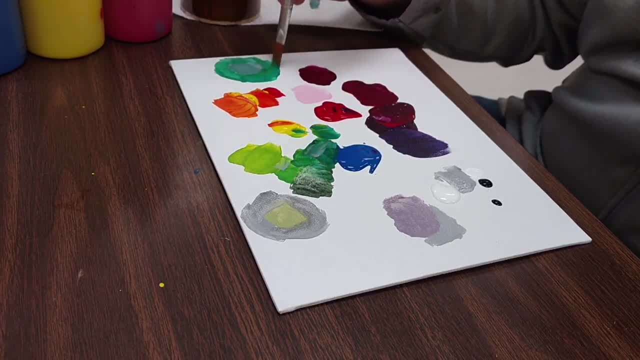 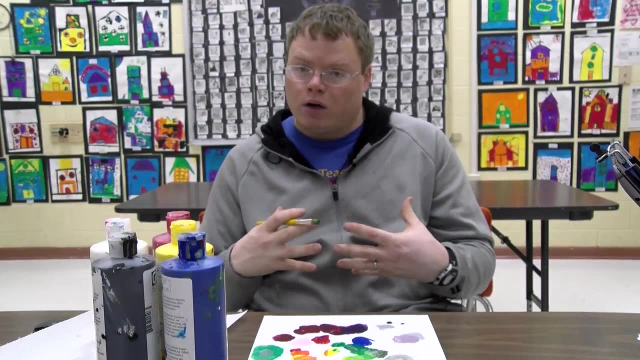 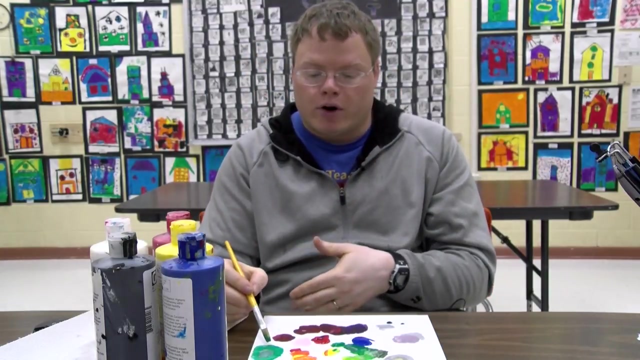 Then it makes that desaturated color look even more gray, Even less saturated, Because, the colors interacting with each other, Your brain will recalibrate to say: Here we have a very vivid color, The one beside it must be gray, Whereas here your brain says: 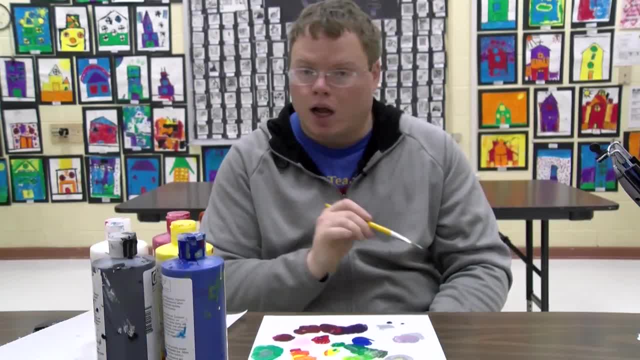 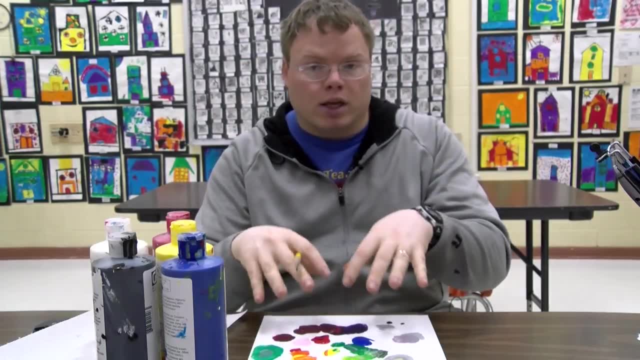 Oh, we've got this gray, The one beside it must be colorful, So your brain will automatically- And that's all done up here in your brain. That's not done here on the canvas, That's done here in your brain As the viewer watching it. 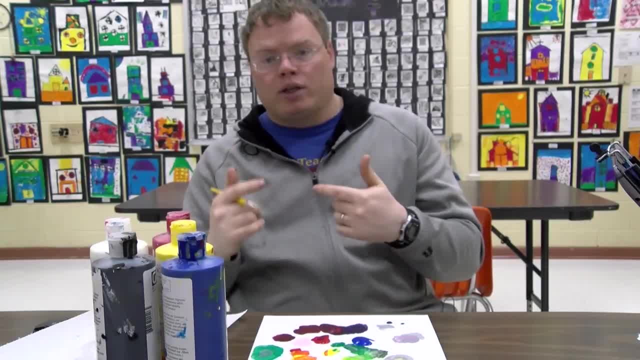 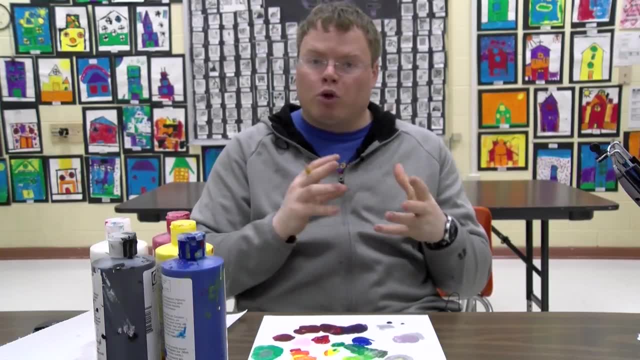 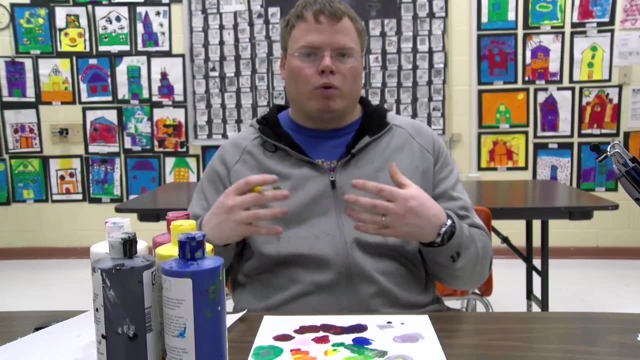 Looking at it, And that's an important thing to know, Because the way that the viewer interprets Art is very different from the way it's mechanically put together. So understanding all of these concepts can help you when you create your artwork. It can help you to make your pictures stand out more, if that's what you want. 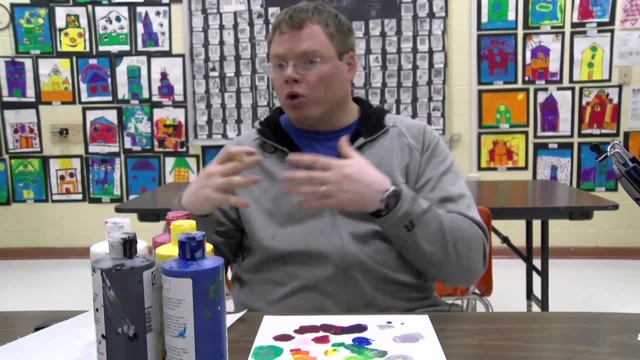 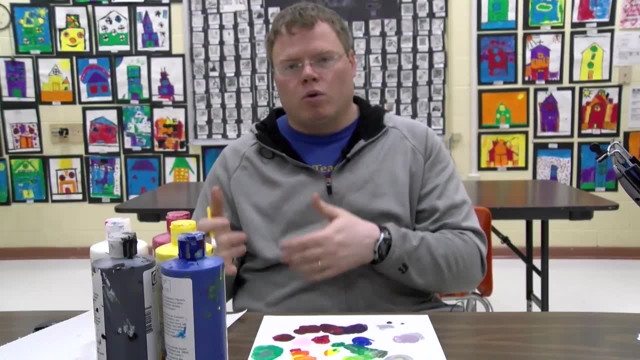 Or make your pictures more unified, if that's what you're going for. So there's all sorts of things that can. That understanding these mechanics can help you in your artwork. Now I would be remiss if I showed you all of this about color. 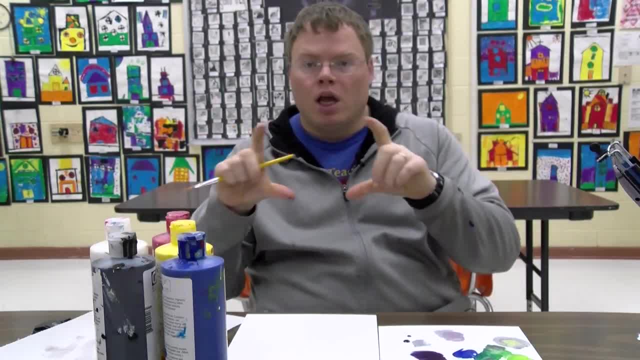 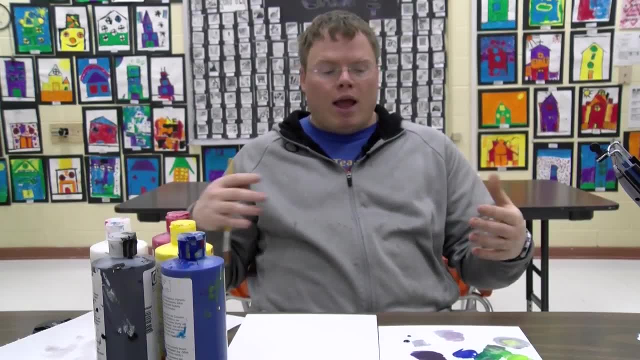 And didn't talk about color schemes. A color scheme is when you choose a very limited set of colors To create a piece of artwork with, And there are lots of different ways to think about a color scheme. You could think about opposites. 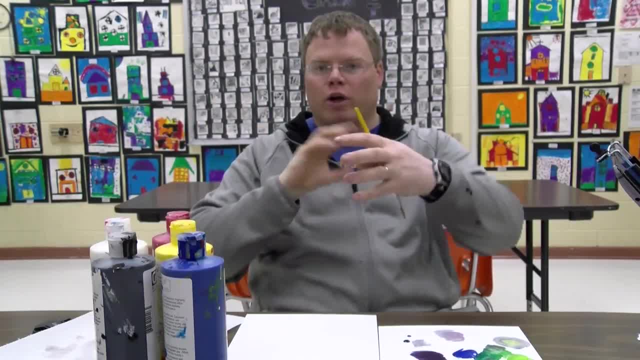 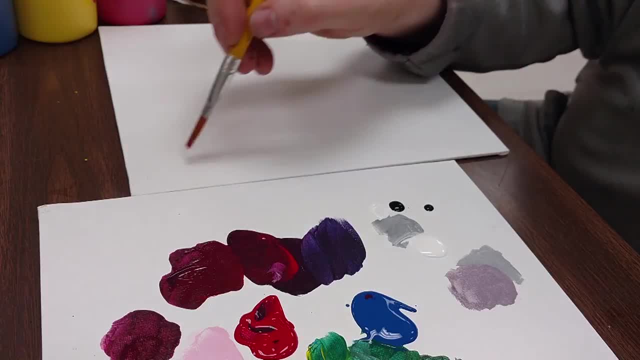 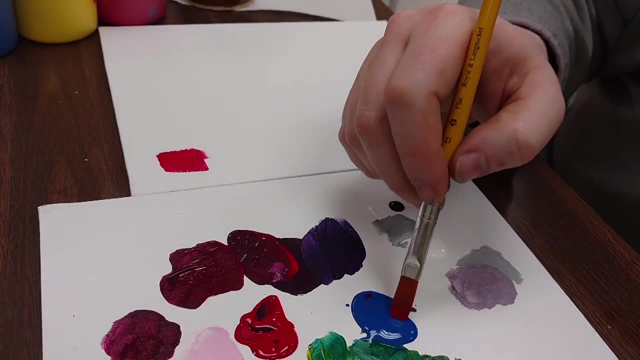 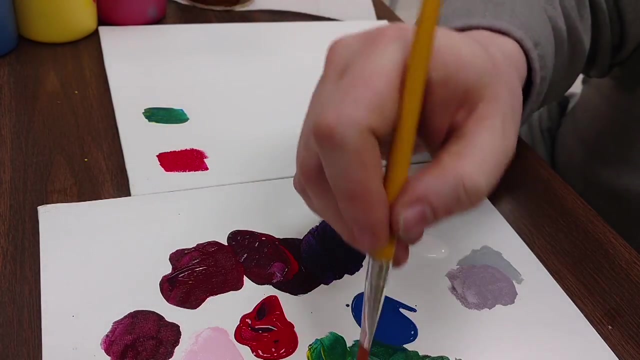 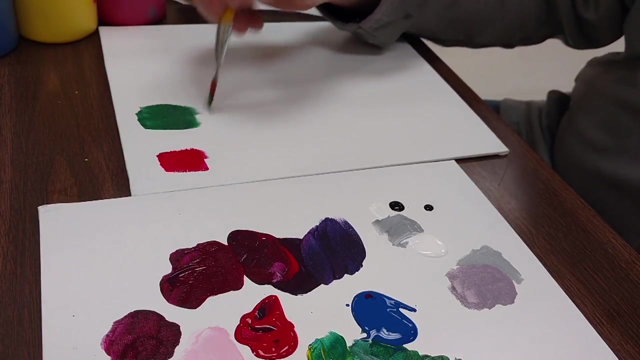 Complementary colors. If you want high contrast, You want your picture to really pop. You could use opposites on the color wheel. So for example, Red And green. Red and green are opposites, But With a complementary color scheme. 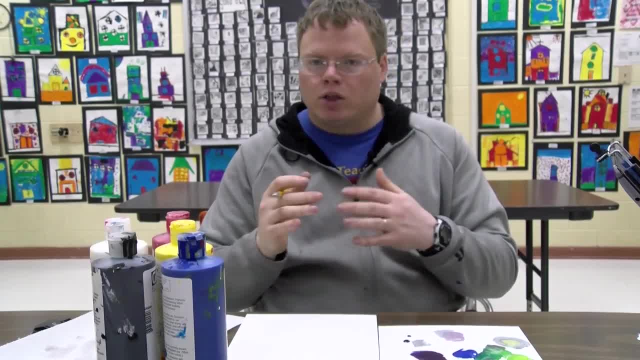 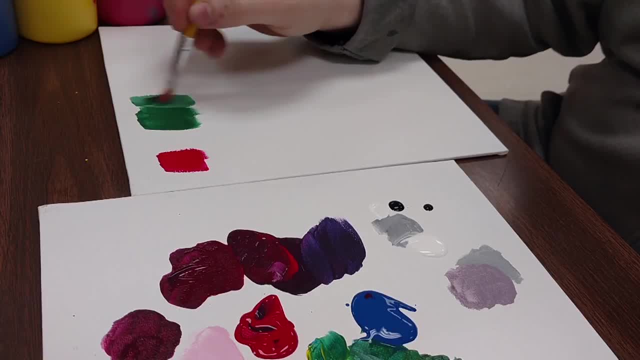 You're not just going to use straight red and straight green. You can use different values of each And different saturations of each. So I could use a really light green, A lighter value of green, Or maybe even a really much lighter value. 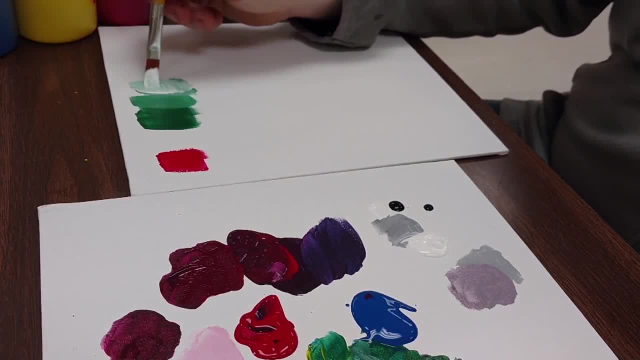 Trying to mix it much, much lighter. There we go. That blue, That blue in the green is a very strong pigment And white is a weaker pigment, So it required a lot of white to make a pale green there. Cleaning off my brush a little bit: 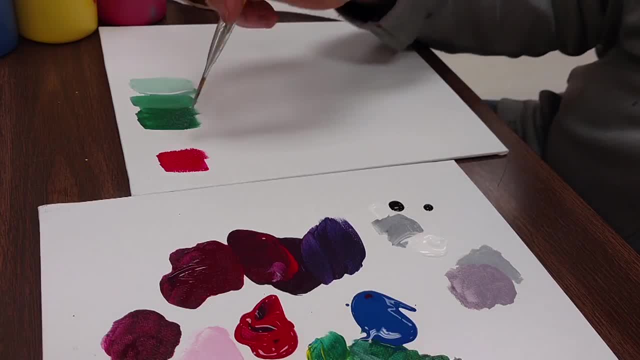 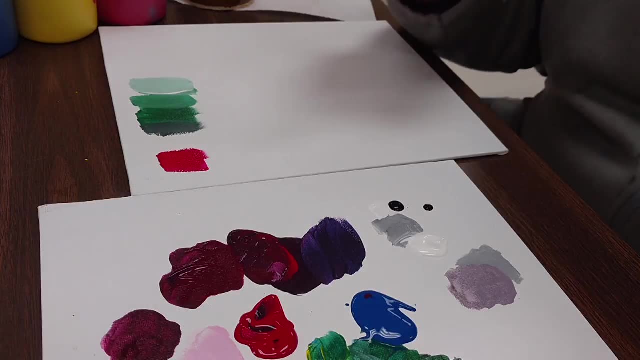 I'm also going to make a darker value of that green, Almost black here And it might even show up as black on that camera. But you know what? I didn't clean my brush very well. That had a little bit of white in it still. 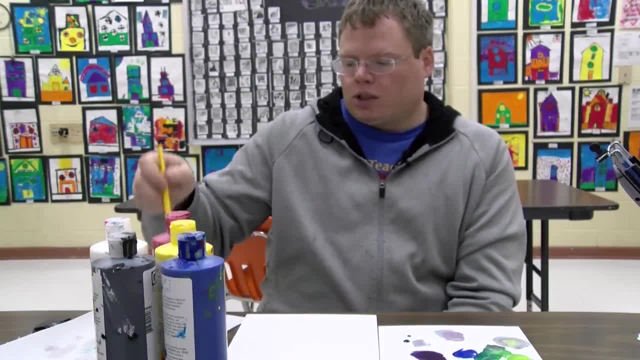 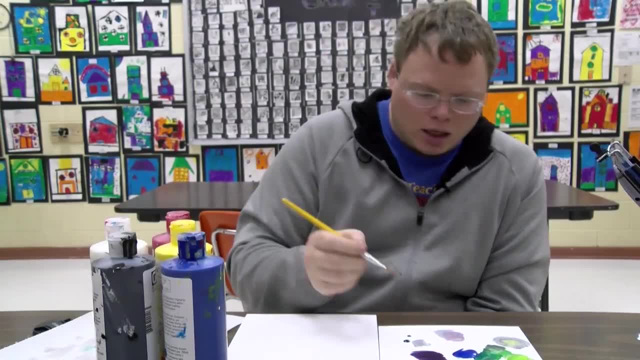 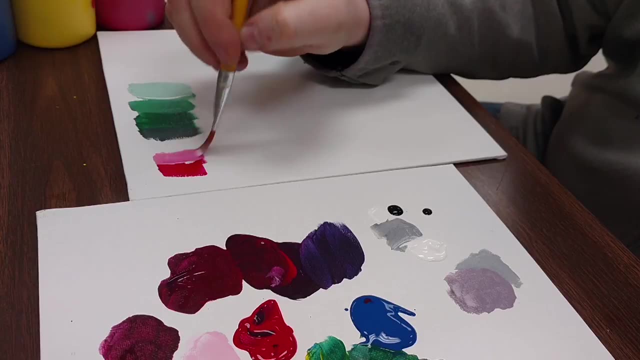 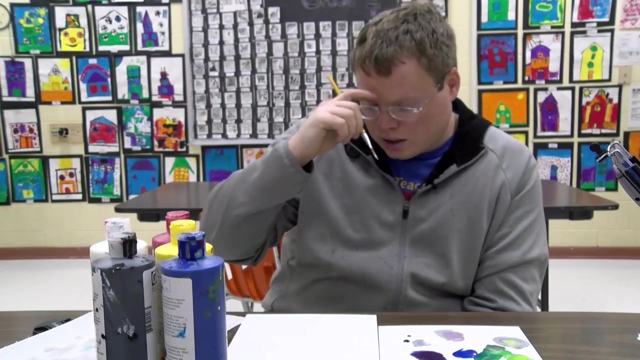 So that made a very grayish green. So Let me clean my brush a little better before I move on to the red And see what happens if I make some lighter reds, Some really light reds, And Maybe I want to desaturate a red with a green. 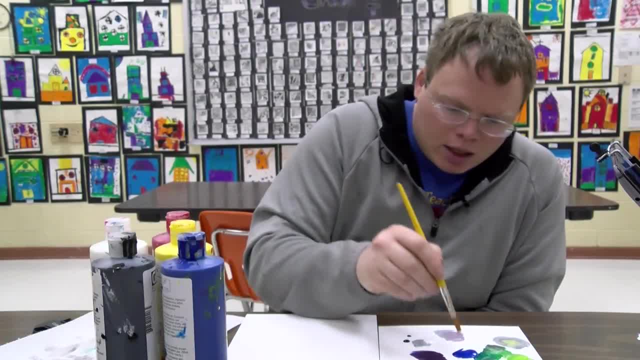 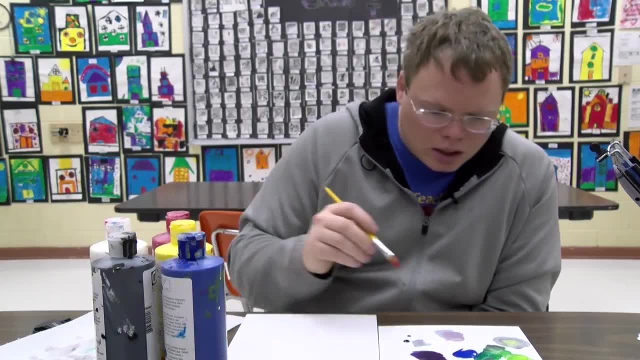 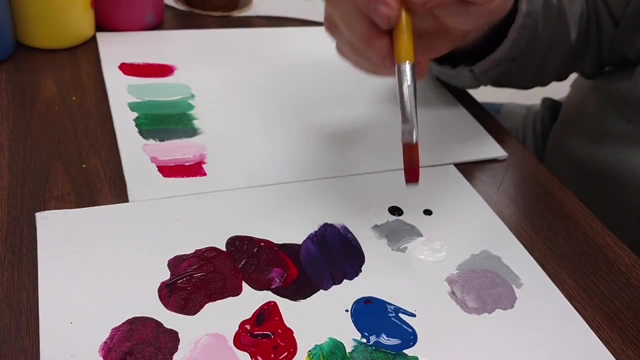 Make it a more neutral red. So to do that, I would take some of this red And Pick up Some of this green over here. I wonder I'm probably getting too much of the blue. It's probably going to look too purple. 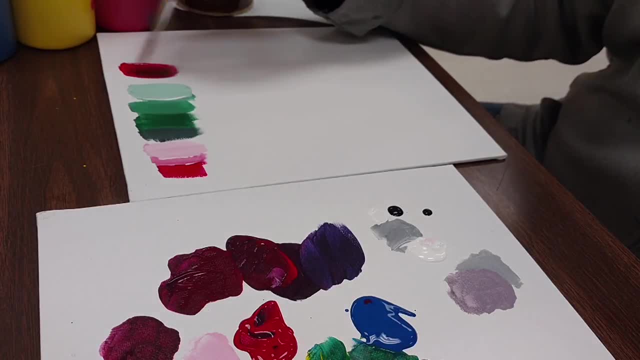 So I need some yellow in there To counter that out. There we go. See, that looks like a very brownish red. Okay, I could make it darker, A darker brownish red, By mixing some black with it. So you see how I can create lots and lots of different colors. 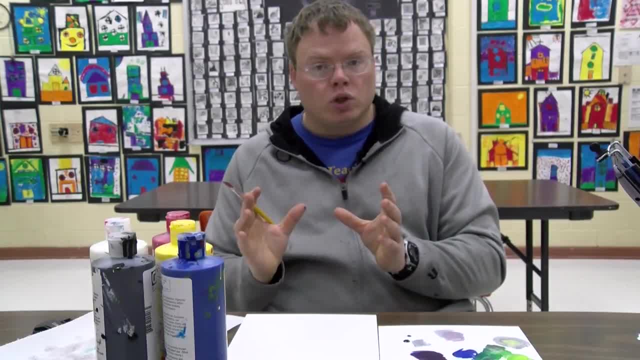 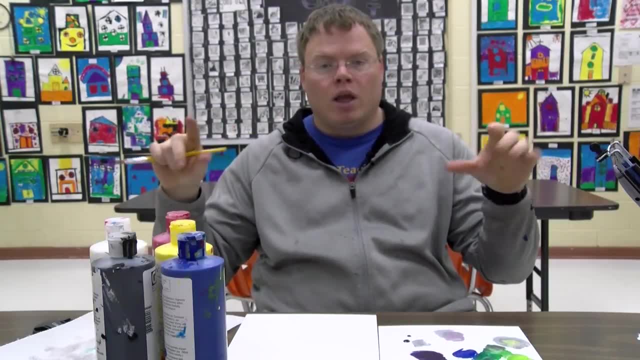 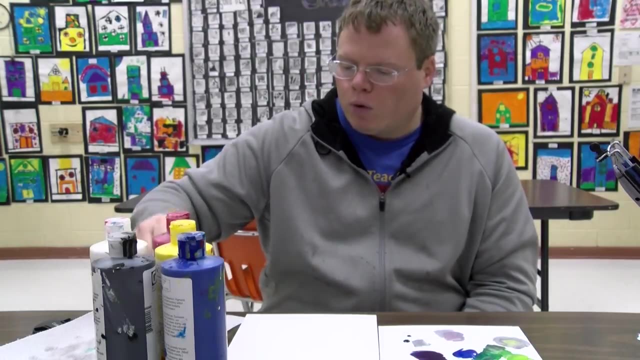 While just using two hues, Lots of different colors, Two hues that are opposites. on the color wheel That means they are complementary, But I'm using lots of different colors within those two hues. Okay, What if I want a picture to be much more unified? 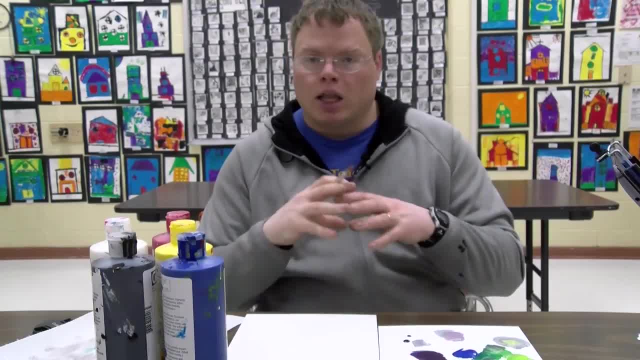 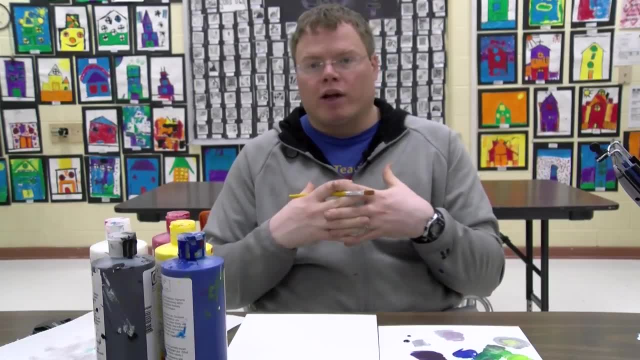 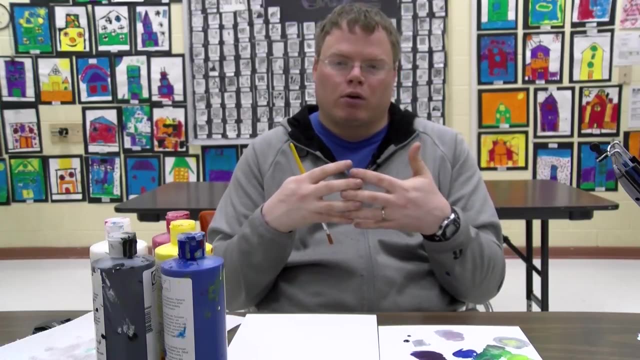 What if I want a picture that has a lot more similarity in the colors, Not as much pop, But more of a unified feel Where everything feels like it belongs together? Then I might go with what's called analogous colors, Which are really close next to each other on the color wheel. 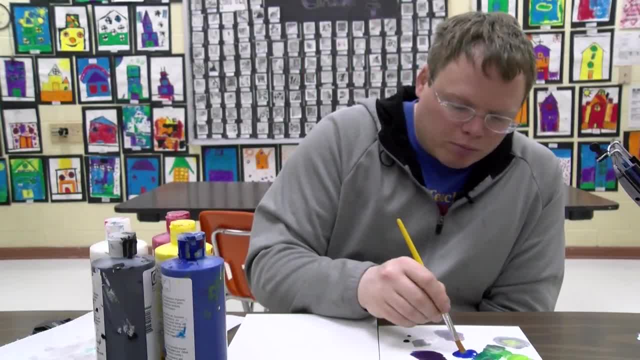 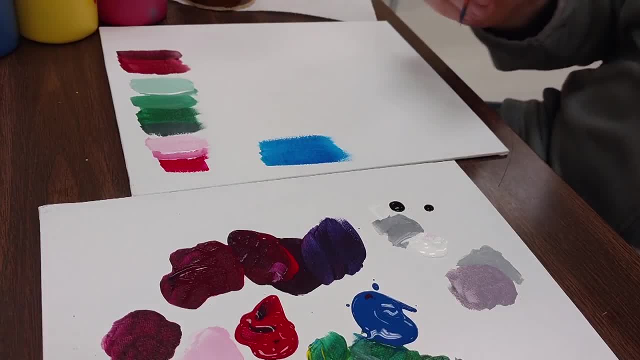 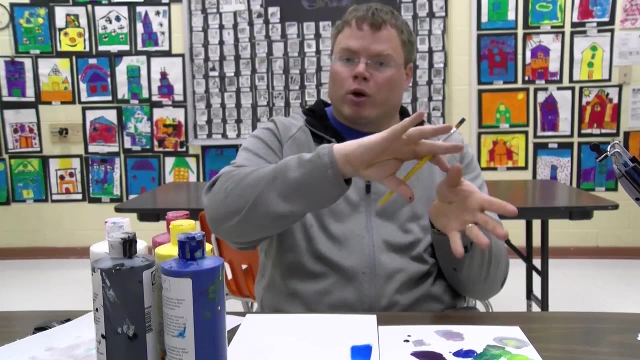 Here's how that could look. Maybe I want to start with blue, And what's next to blue? You could go either way on the color wheel, Maybe violet and red, Or maybe yellow and green, Or maybe blue with yellow. I'm sorry. 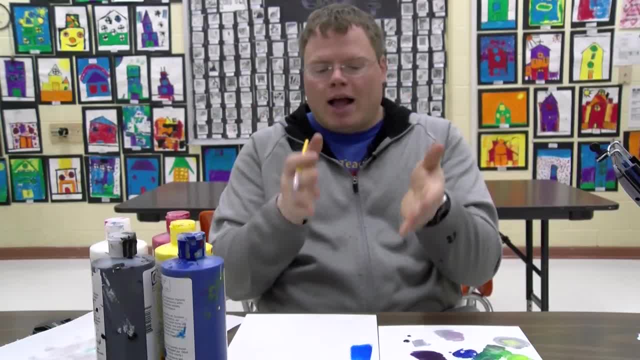 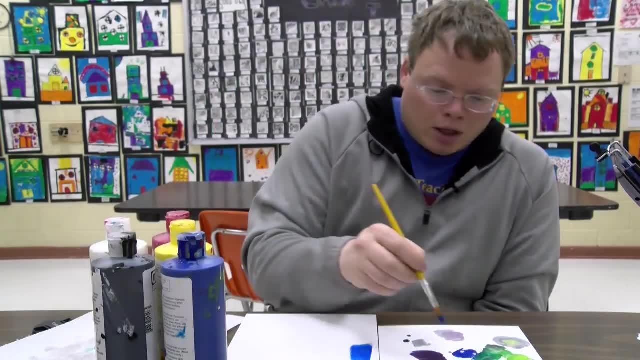 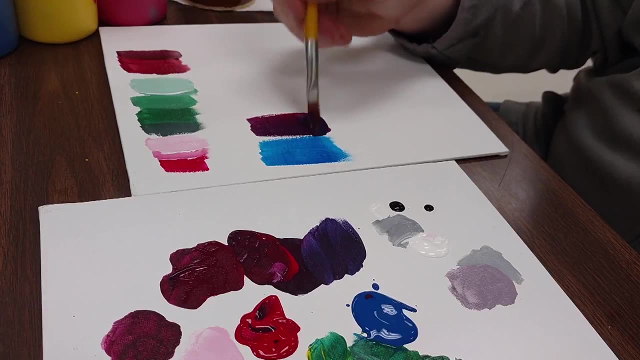 Blue with green on one side and purple on the other. I think what I'm going to do here Is go from blue to purple, Maybe on into the red side of the spectrum, So making a purpley color, And I can do different kinds of blue and different kinds of purple. 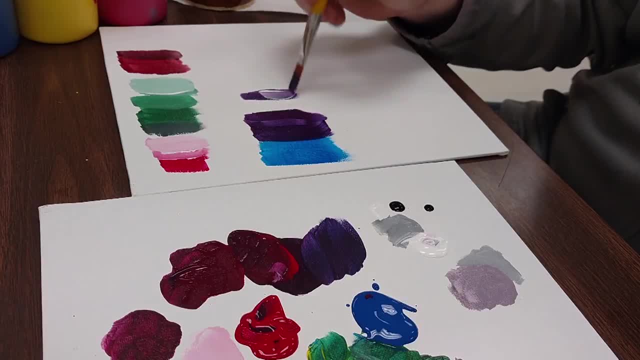 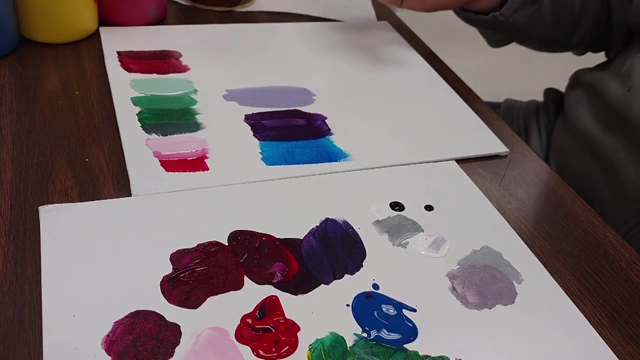 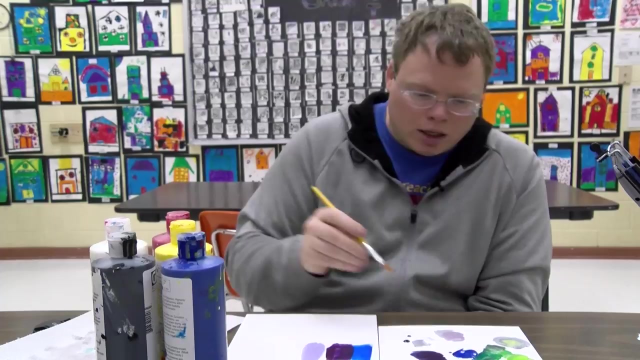 So while I've got that purple on my brush, I might mix it with some white To make a lighter, more lilac kind of color, A turquoise, A desaturated pale purple. I might clean my brush here And make a really reddish violet. 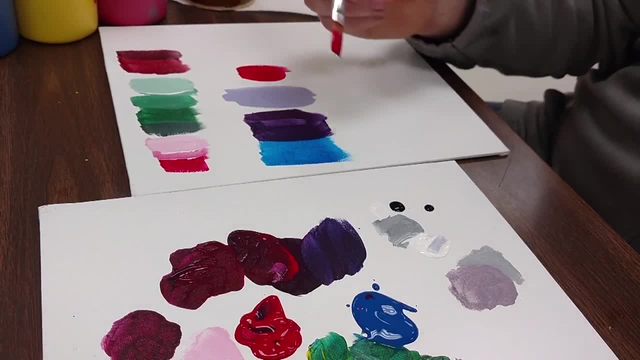 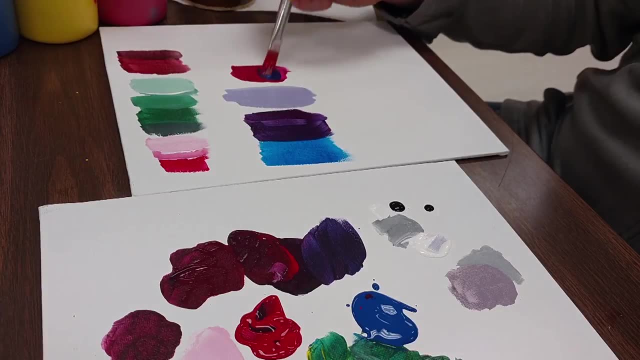 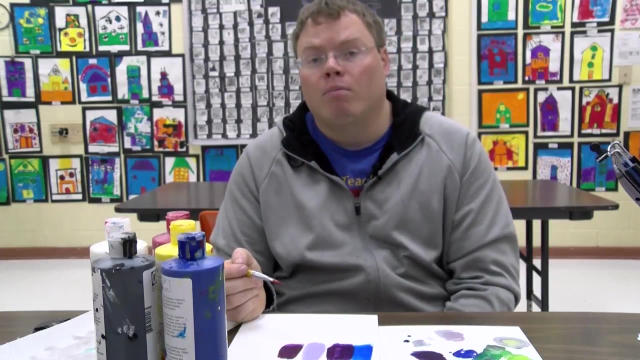 Use a whole bunch of that red With just a tiny touch of that blue To make a really reddish purple. Maybe a little bit more of the blue in there. That's too red for my analogous. That was too much. Blue is a very powerful pigment. 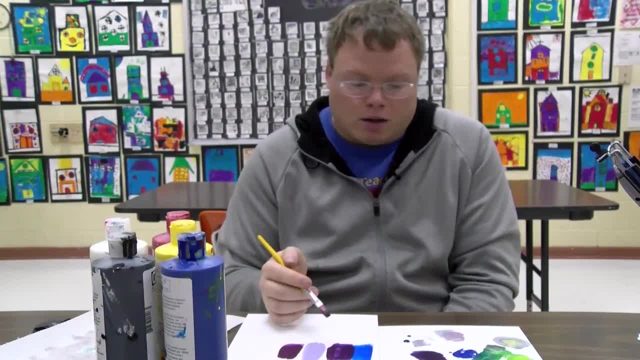 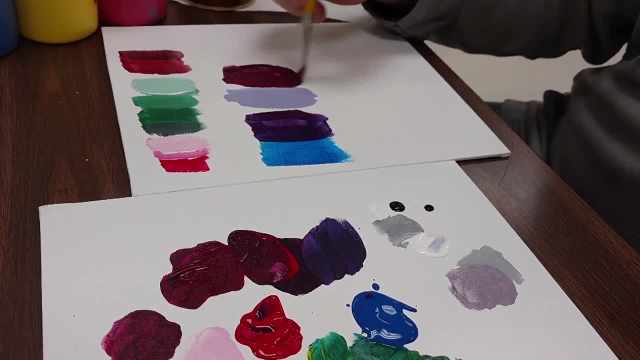 If I didn't already say that It just overpowered that And made it look basically like that one. So I need a bunch more red To red that. up There we go. Red, violet- Okay, So you can see the difference between that color and that color. 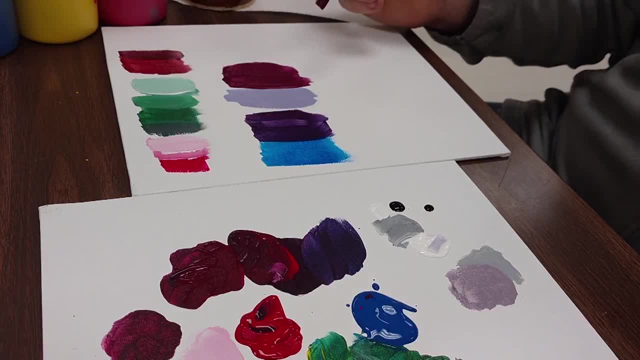 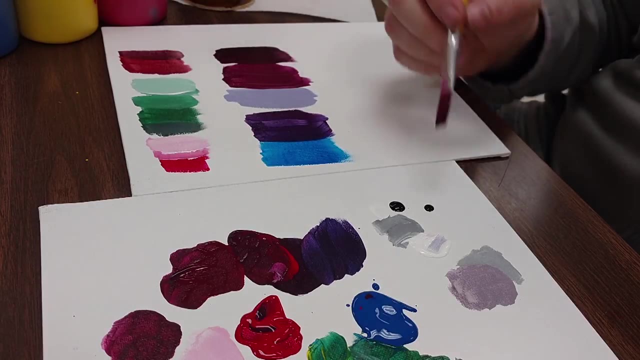 They're different hues. One is more red, One is more violet, Red, violet and violet. Now, This I could make a darker version too, So let's get a little black in there. Make it a dark reddish violet, Maybe make a desaturated version of it. 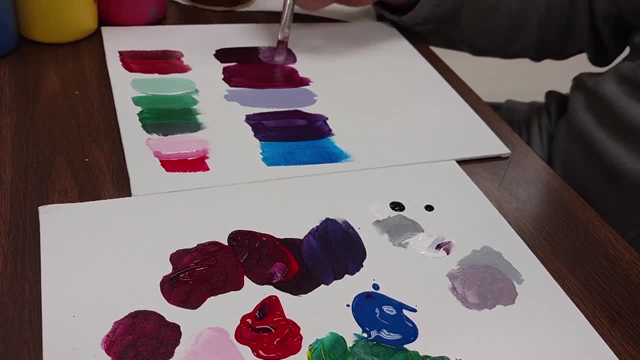 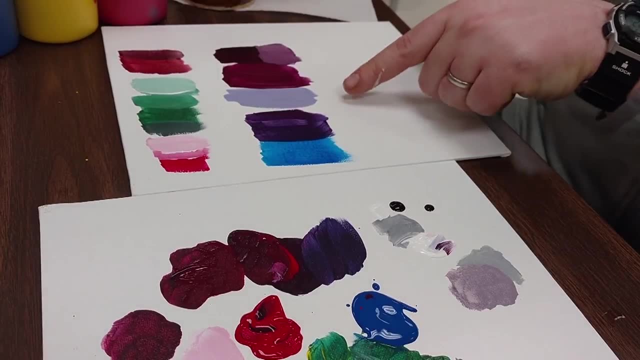 By adding a little white to the black one, So it's sort of a grayish red violet. Okay, So you can, And then I can play around with the blues too. I've played with the purples a little bit. Let's play with the blues next. 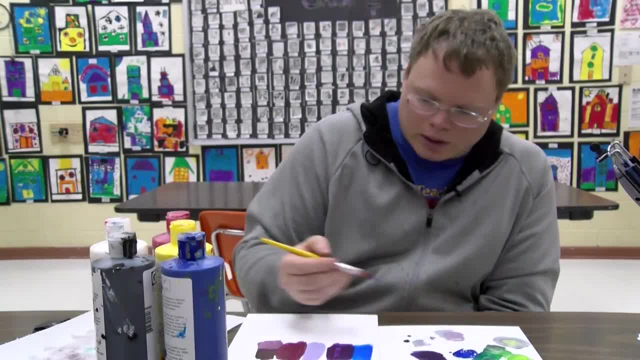 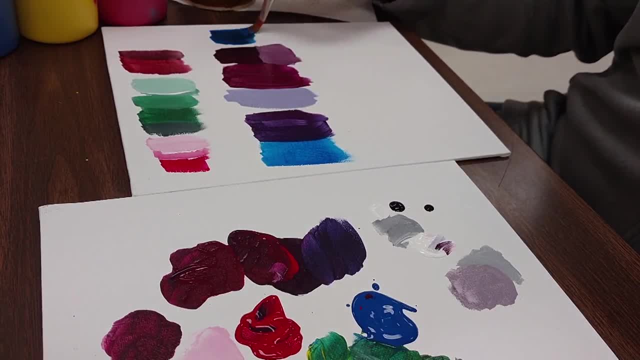 Maybe I want to make a really really dark blue, So I'll start with a bit of blue. Black is really strong, It kind of. It doesn't take much black to really darken up a color, See. So there I've got a darker blue. 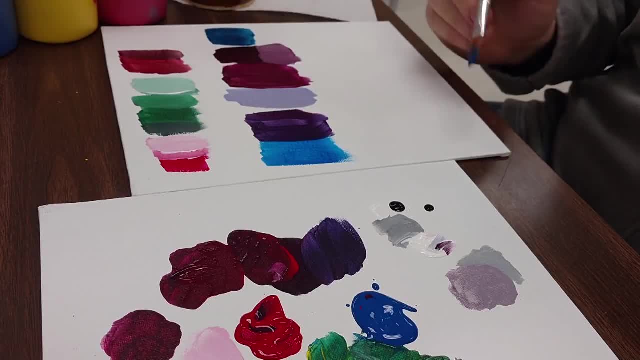 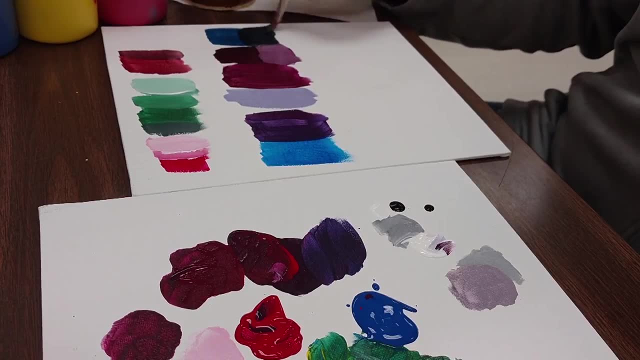 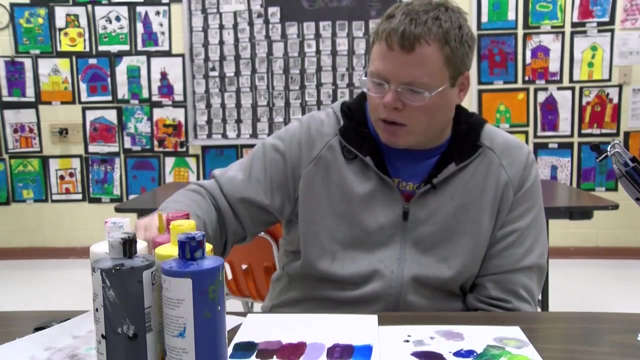 Maybe a little touch darker than that. Maybe I'll make one that's even darker blue. That's like a midnight blue, So dark That you can barely tell it's blue. Okay, Maybe I want to have a lighter blue. Let's wash my brush. 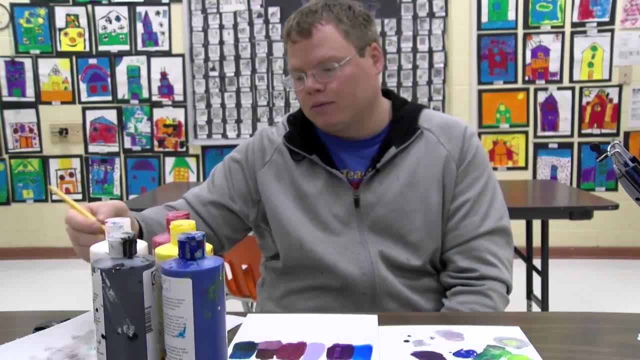 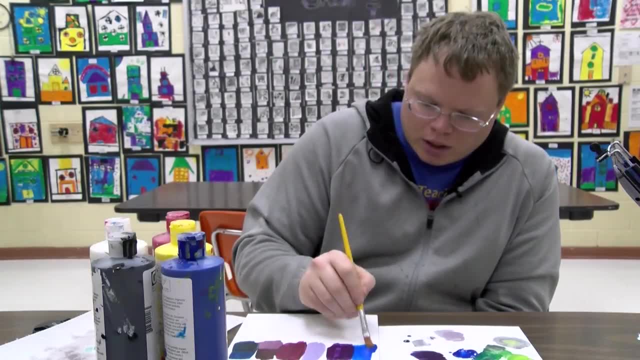 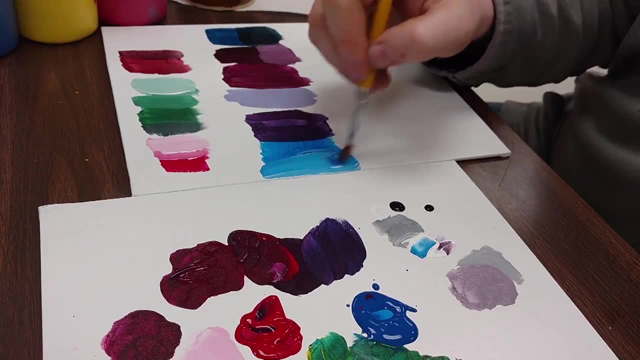 Let's wash my brush to get all that black out And let's make a lighter blue By mixing some white and some blue. It'll be kind of like a sky blue if I can get enough white in there. There we go, Starting to get there. 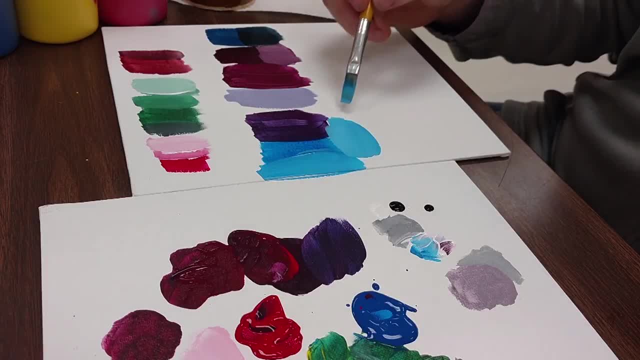 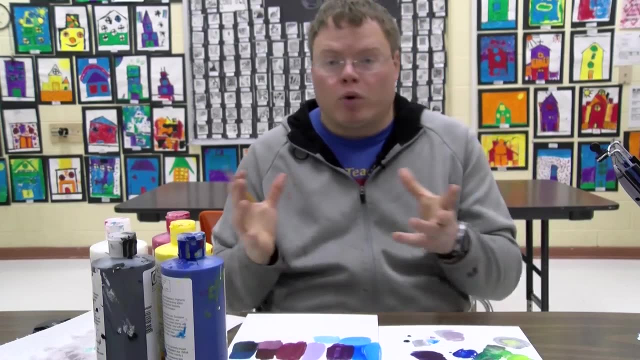 And so here, these colors all feel like they belong together. They're very similar to each other. Every one of these colors, They all have one thing in common: There's blue in all of them. Right, Even these purples. To make a purple, you have to add blue. 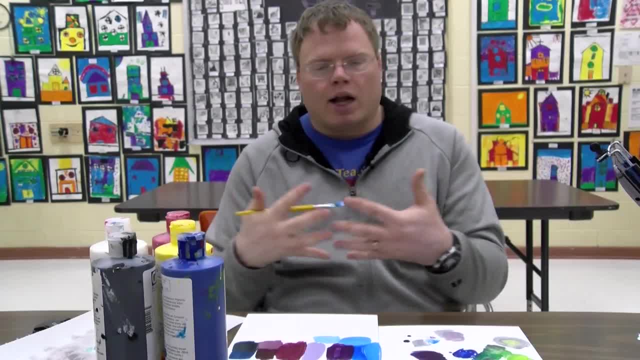 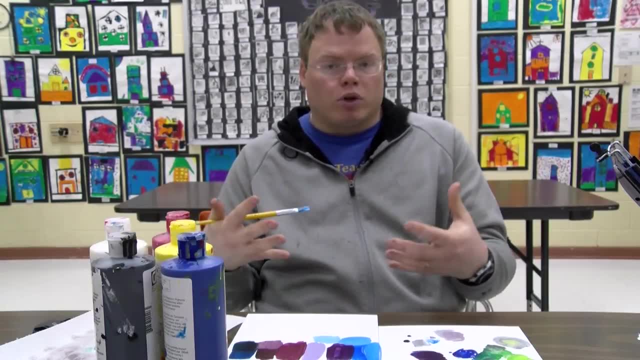 Right. So all of these have blue in them, So they've got a common thread that binds them all together, And using these colors together would really make it feel much more unified. And here I've only got blue and purple- Still, basically just two colors. 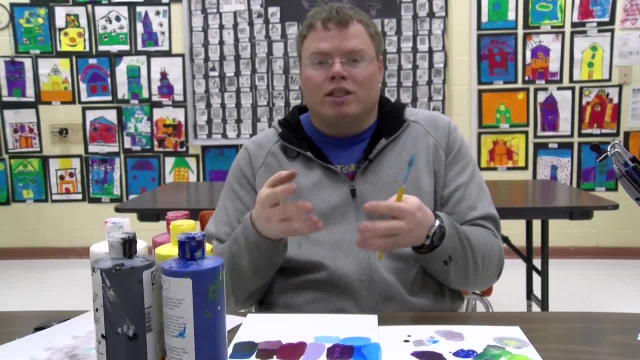 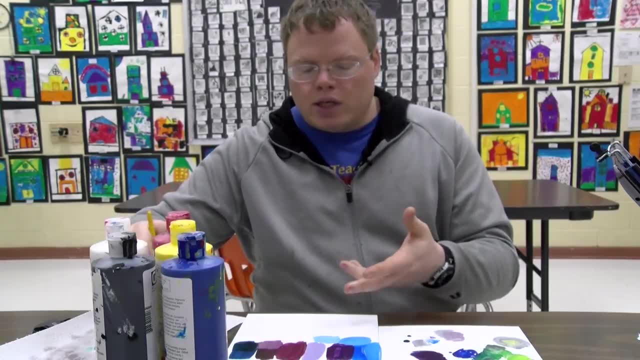 Maybe you could say: red violet is my third, But I'm using. Those are the hues that I'm using, But I'm making lots of different colors out of them. Now, these are the most common ways to create color schemes, Complementary and analogous. 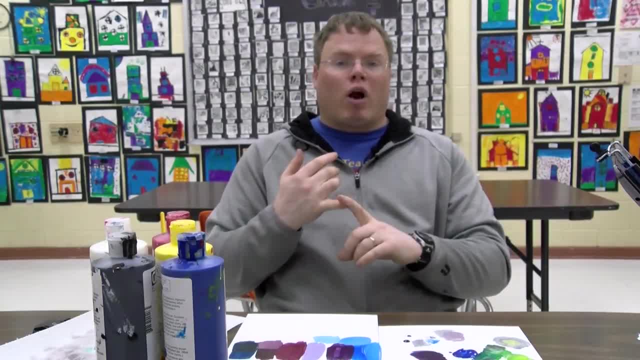 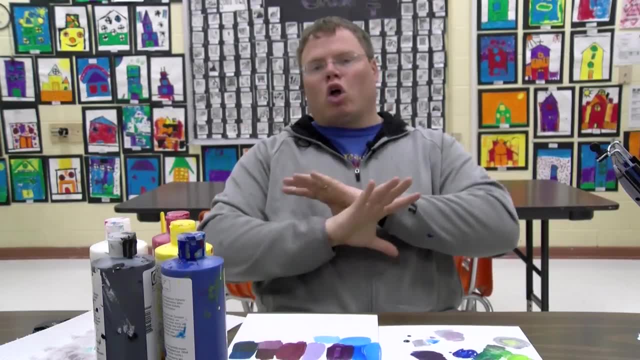 But there are tons of other ways to create color schemes: Triadic, Where you make an equilateral triangle on the color wheel. Tetratic, Where you make a square or a rectangle. There's all sorts of different ways- Split, Complement. 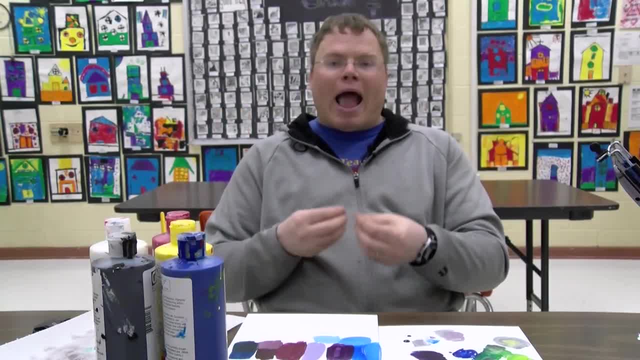 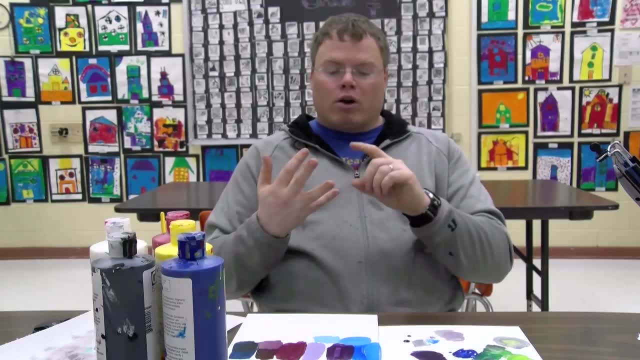 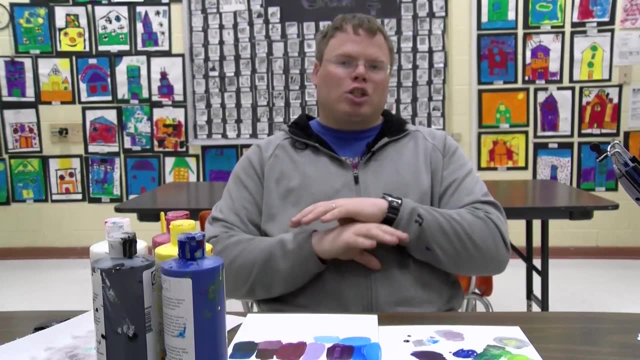 But Understanding the basics first And how to put colors together And how to create different colors using the same hues, Or how to create different hues, Different saturations, Different values of your colors. Understanding all of that And just playing with it. 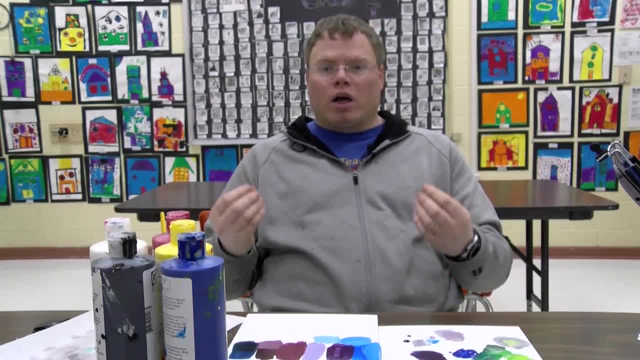 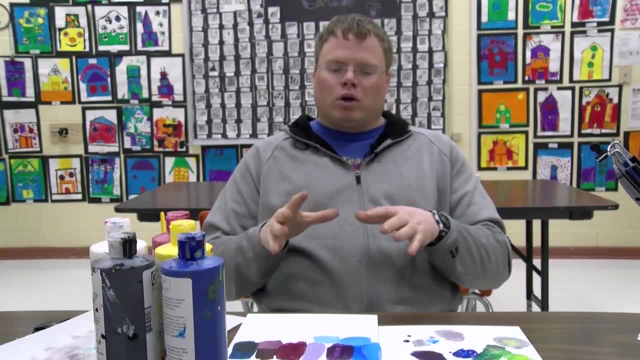 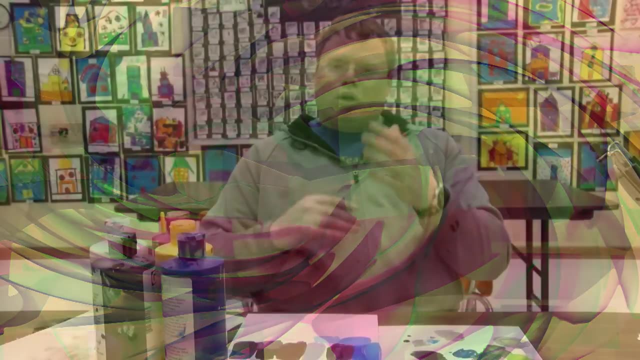 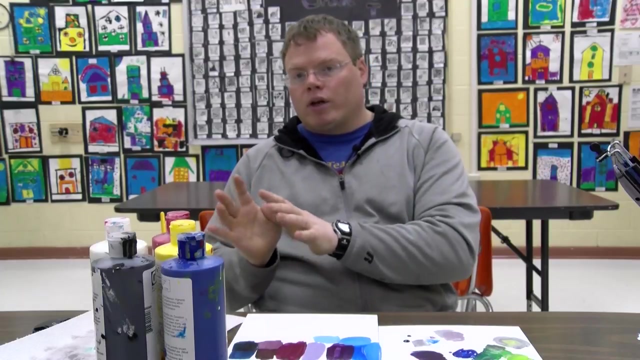 Can go a long way to helping you understand how color itself works. Now, In your artwork, I would encourage you to start by playing Making some color studies to see how these colors interact together, And then start limiting yourself on your colors, Instead of trying to use descriptive colors to show exactly what color something really looks like in real life. 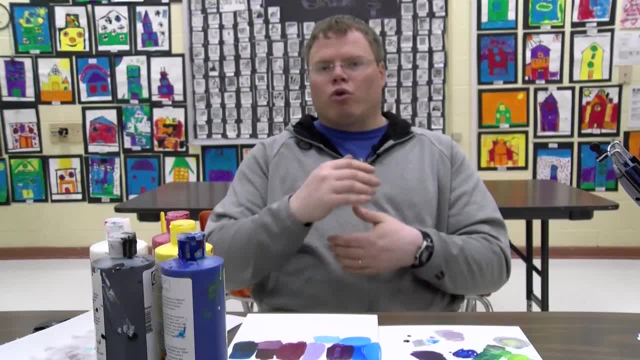 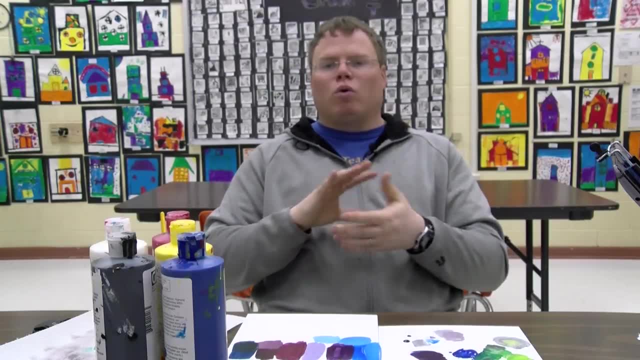 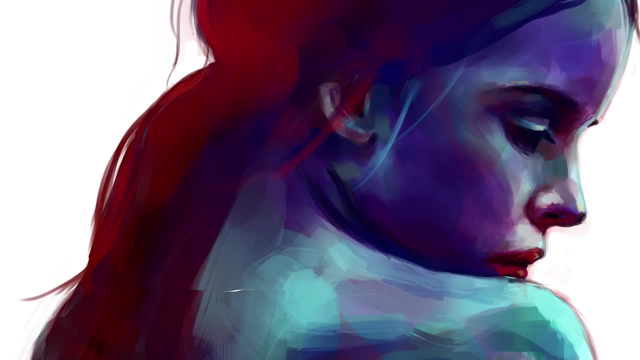 Start manipulating those colors to create more of a visual impact. Whether it be a pop or a unification Or somewhere in between, There's a lot that color can do. Sometimes it can be expressive emotionally: Blues could be more calm or more sad. 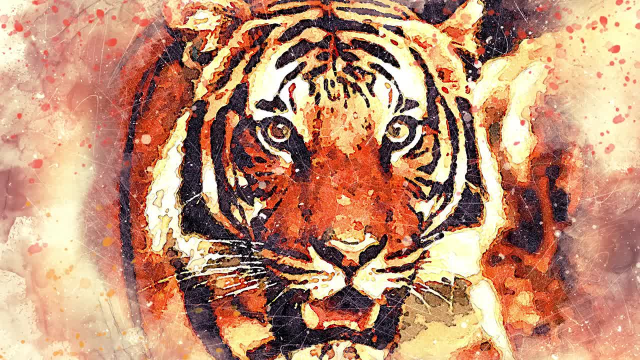 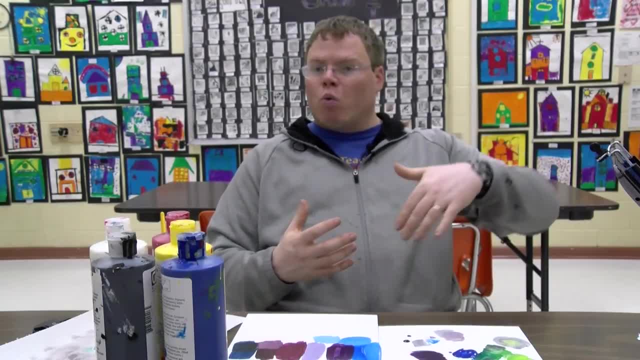 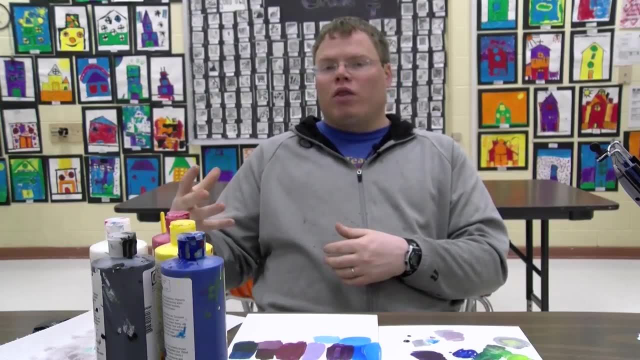 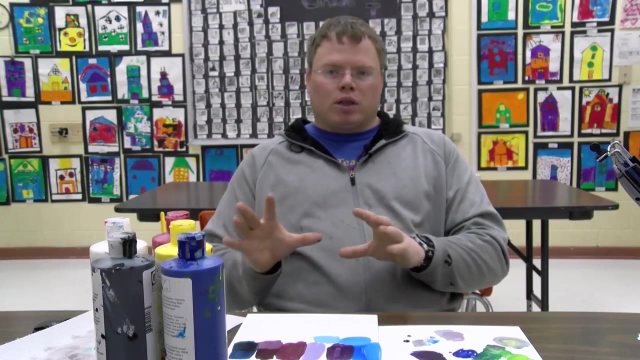 Warm colors could be more exciting, More vibrant, More lively, More passionate. Generally speaking, The warmer the color, The more powerful and strong the emotion. The cooler the color, The more calm and relaxed the emotion, Not always, But generally speaking. 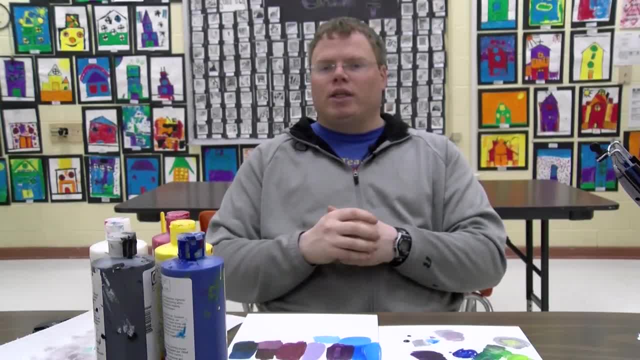 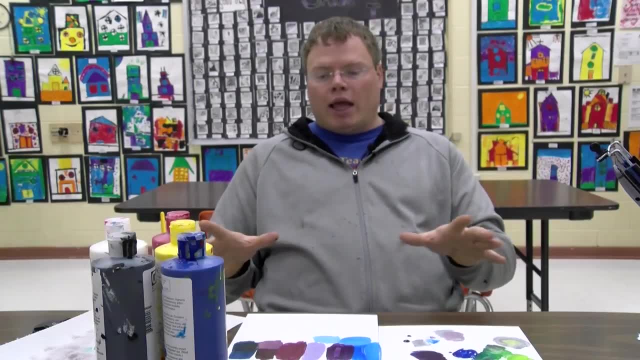 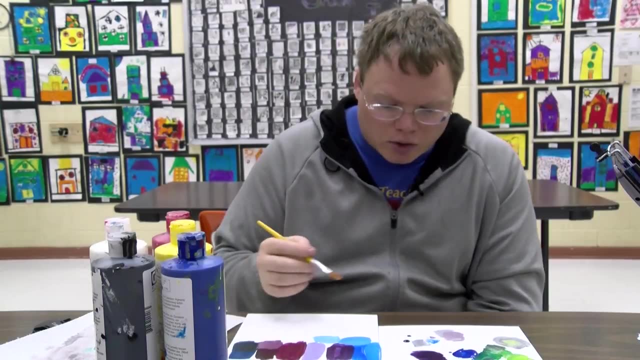 Also, the more vibrant the color, The more saturated the color is, The more powerful that emotion is, And the more desaturated it is, The more calmed down it is. So an example of that Would be: If I want a color that's really passionately loving. 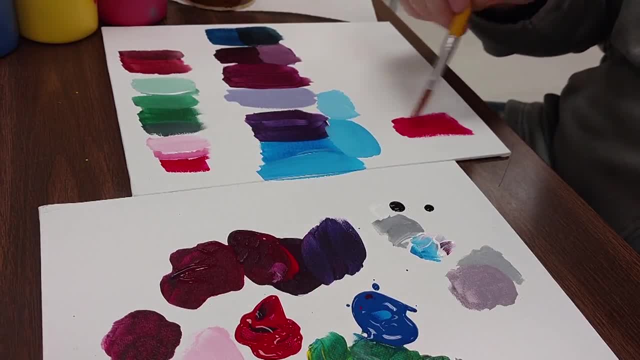 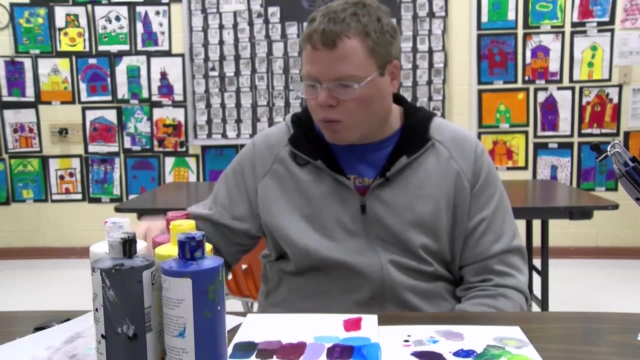 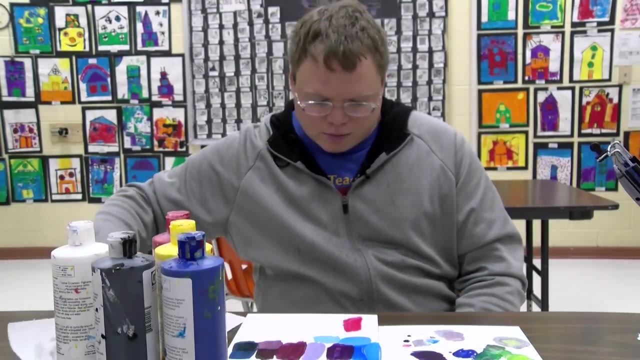 Really, You know You think about pink when you think about loving. The more saturated that pink is, The more strongly loving it will be. I need more white. I ran out of white over here, So right away that red by itself. 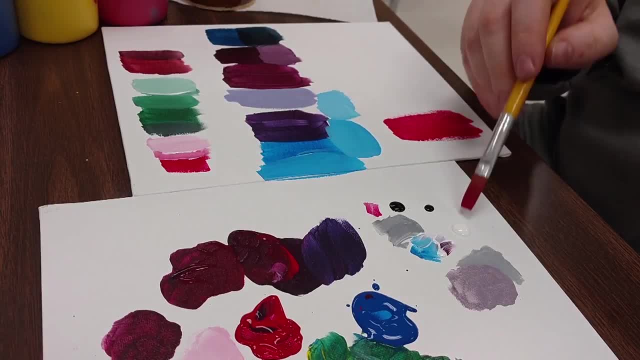 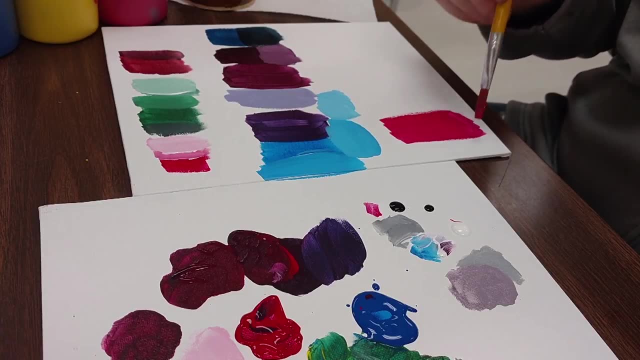 Is pretty dead gum, Powerful and passionate. If I mix up a pinkish version of it And make it a really saturated pink like this, With just a little bit of white added, That's going to be a much stronger, More passionate feeling color. 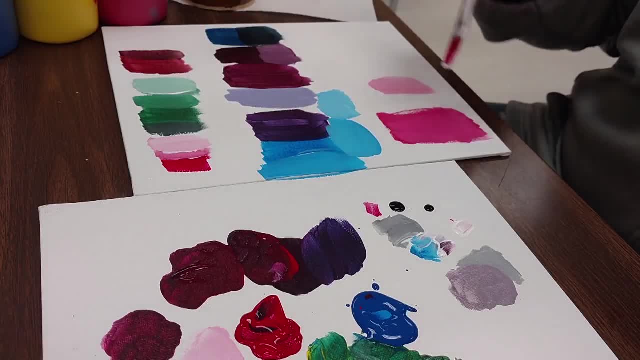 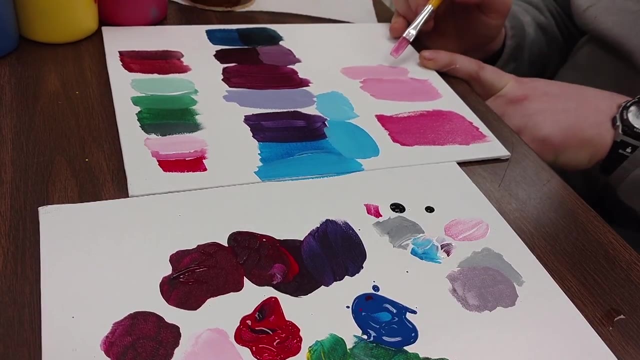 Than it would be if I really desaturate that color With a whole lot of white. The less saturated that color becomes, The less, The more calm it becomes. Now it feels more like a relaxing Still. Maybe it still has that loving. 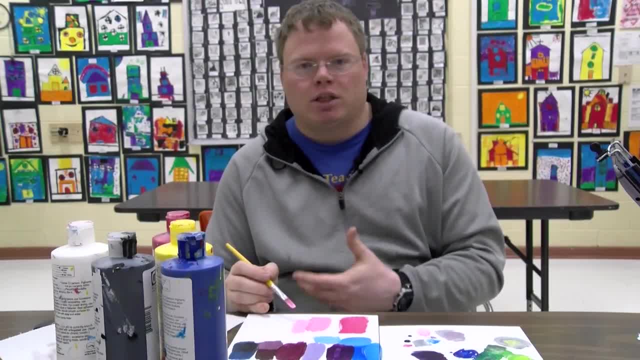 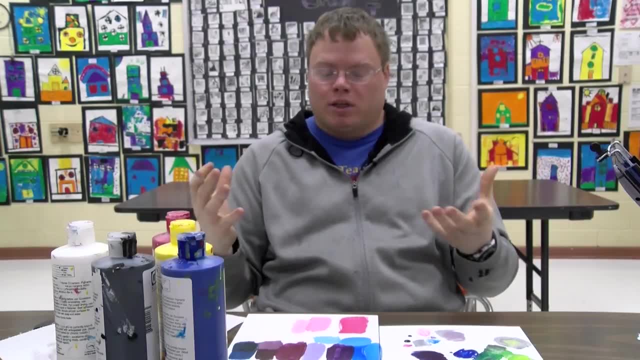 Caring feel, But it's. It's not a passionate loving feel, It's more of a Hey, I love you Instead of this, Which is: I love you, You get the, You get the gist. So the same could be said. 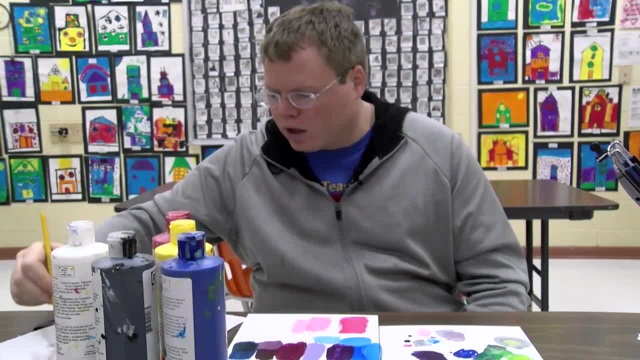 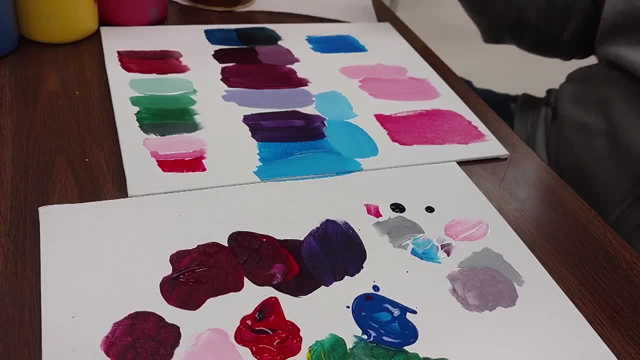 For Any other color, Like if I did a blue You know You think about. I've got the blues, This deep Dark Blue, And especially if I make it even darker with a black Feels really Dreary. 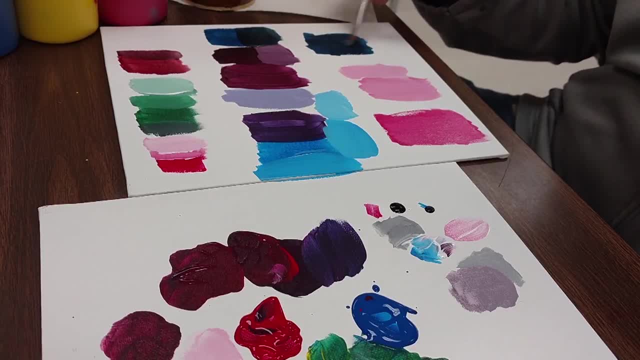 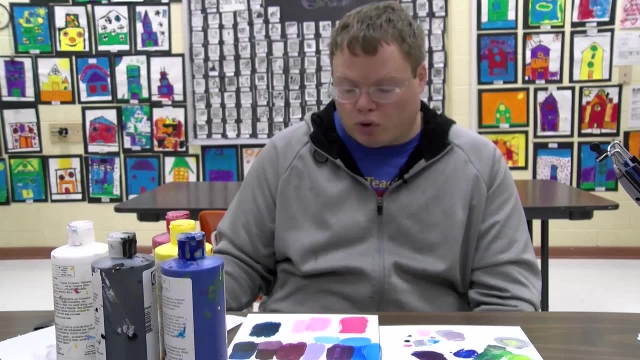 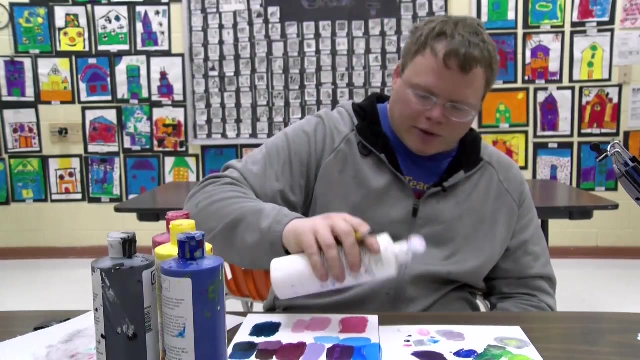 Dismal: Dark, Dreadful, Lonely, Sad, Depressed. If I desaturate that I ran out of white again. If I desaturate that again By mixing in some white, I've still got the black in there too. 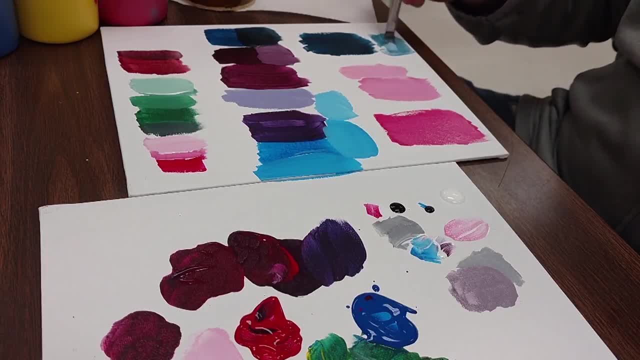 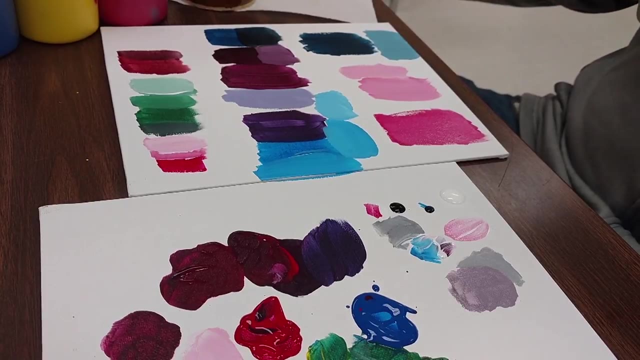 So it's grayish blue. It's going to be much calmer. Might still feel sad and lonely Because it is still A darkish blue. It's not a very vivid blue, It's not a. It's not like a sky blue. 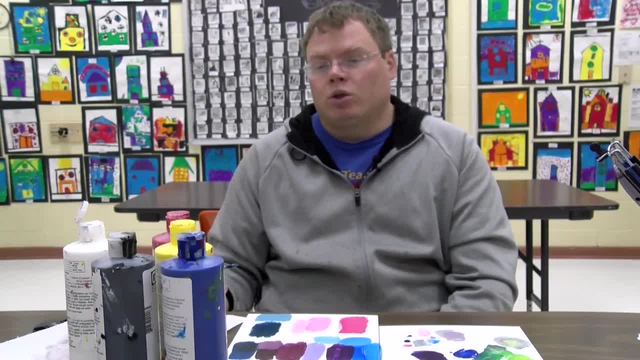 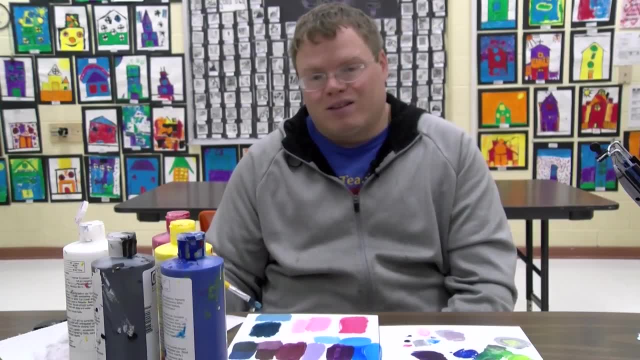 Because it's It's grayed out So it doesn't have the calm blue feeling Like a, Like a sky blue would Or a baby blue Still feels kind of lonely, But it's more like a. I don't want to get out of bed today. 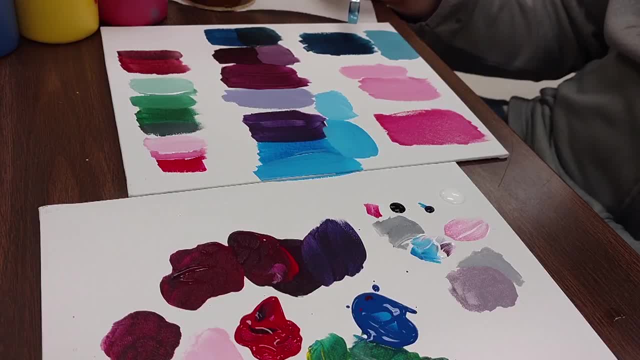 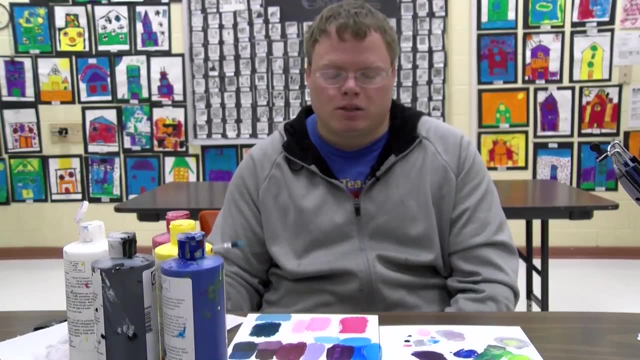 Kind of feeling, Whereas this Has the I really Just, I just I just Don't Wow Kind of feel. Does that make sense? Anyway, I could go on and on forever. I could take hours and hours to explain more and more and more. 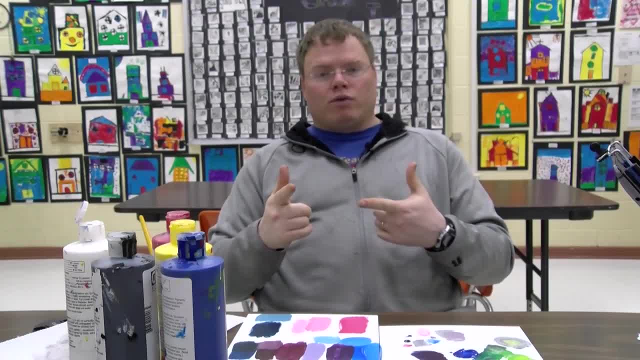 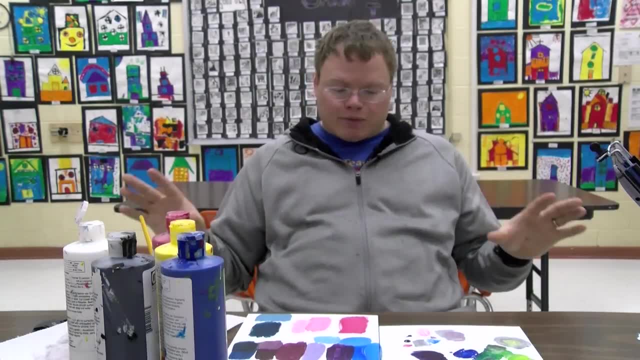 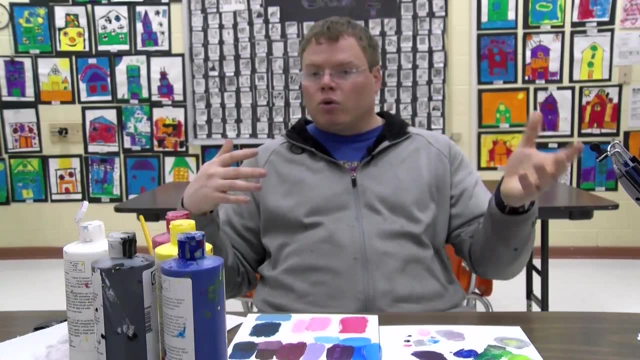 But I think the most important thing for you as the viewer Is to just play with it. Start creating. Take everything I've said here And start making different colors, See how they work together And play on a canvas like this- Or maybe you use colored pencils or oil pastels or something instead. 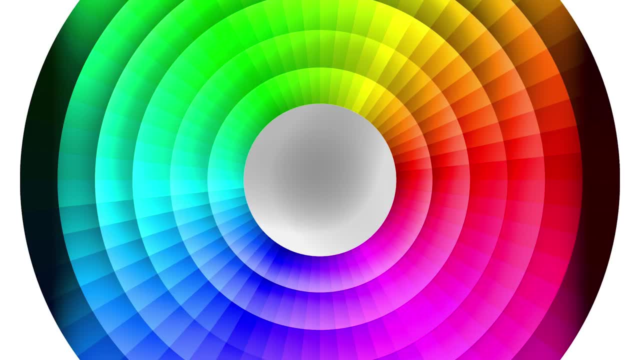 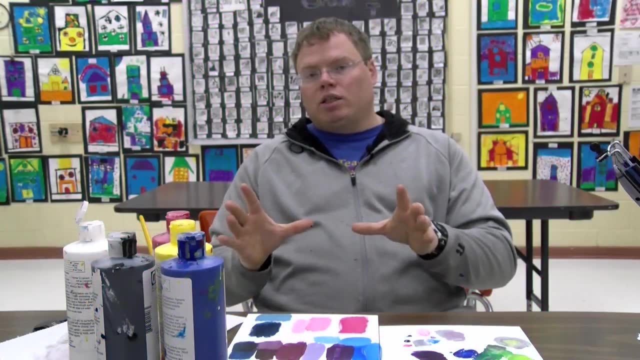 Whatever materials you use, I would say start by making a color wheel. If you want to know how, I've got a video on that, Link in the description. Then Start making color studies. Just play with the colors, Put them together.